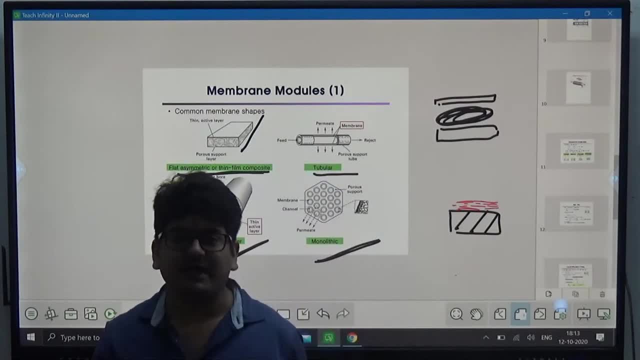 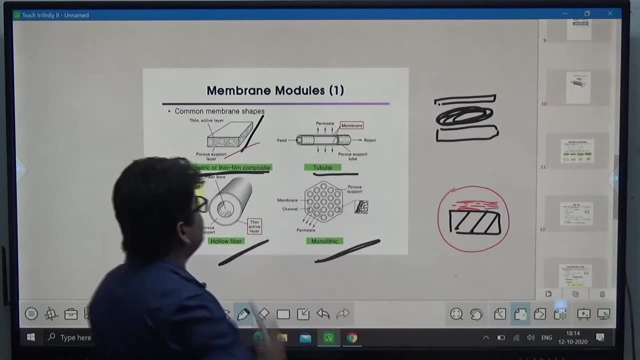 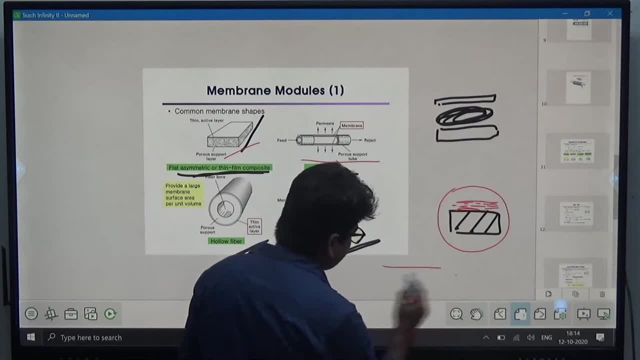 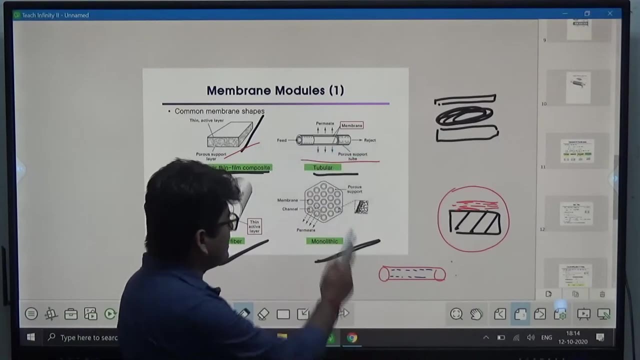 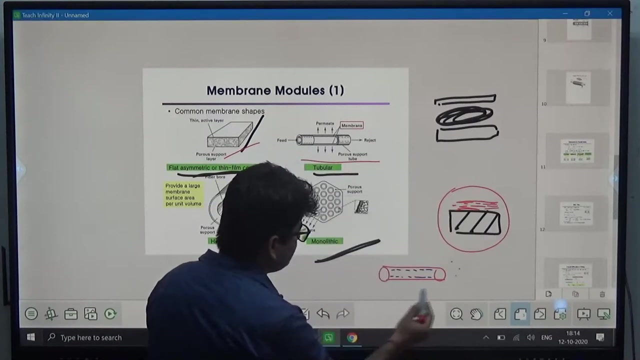 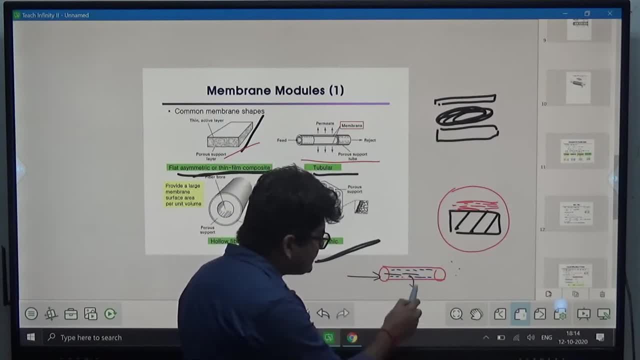 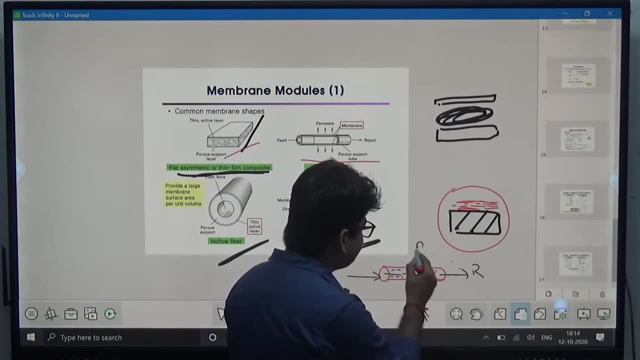 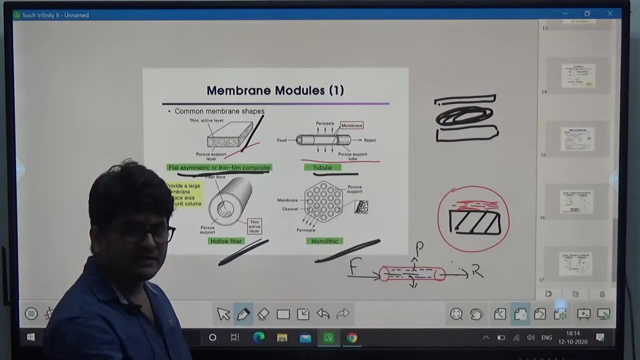 passes through these membranes, so permeate, crosses these membranes, and here we are supposed to get the residual, or you can say the retentate part. okay, this is the tubular membranes. similarly, holofiber membranes are also like that, okay, only the difference is between the working. 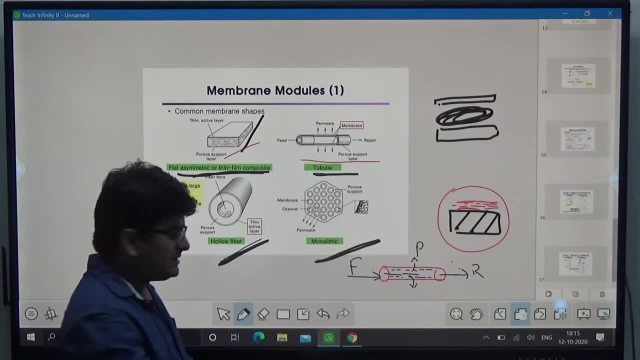 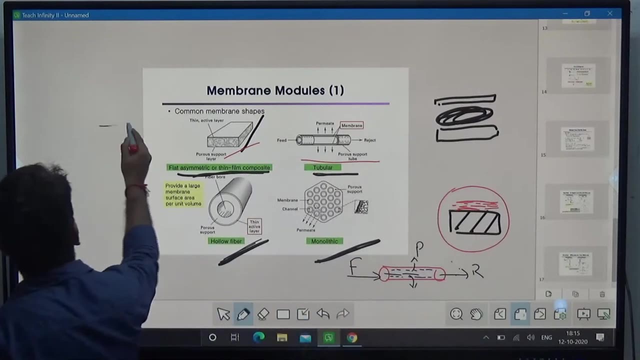 of holofiber and tubular membranes is almost same. the difference is in their size. what is that that we will discuss? and last one is the monolithic membrane. okay, monolithic membranes, you can say a kind of a hexagonal membranes. There we have one hexagonal like this: if you have heard about the shell and tube heat. 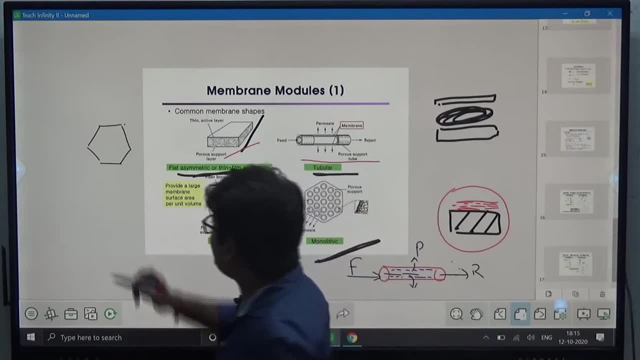 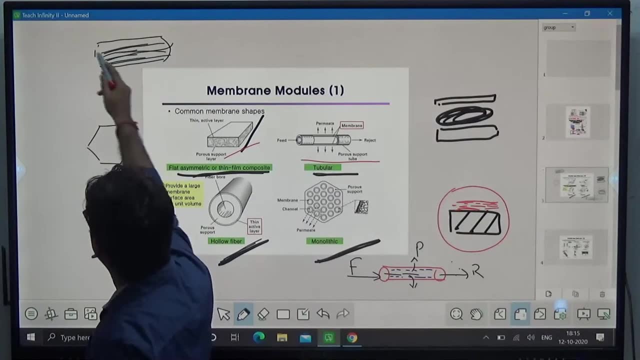 exchanger. so you know that in shell and tube heat exchanger what happened? there is a cylindrical shell and in that shell we have n number of tubes. okay, that is shell and tube heat exchanger. one fluid passes in the shell, one fluid passes in the tube. 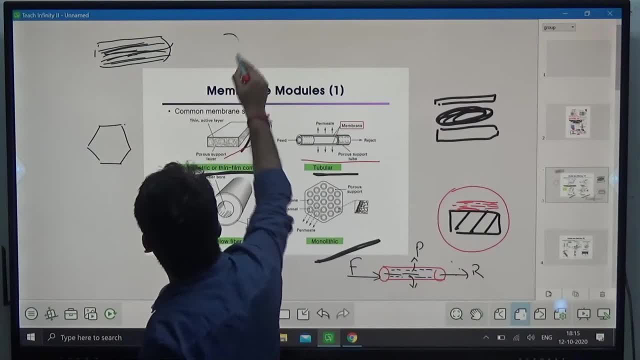 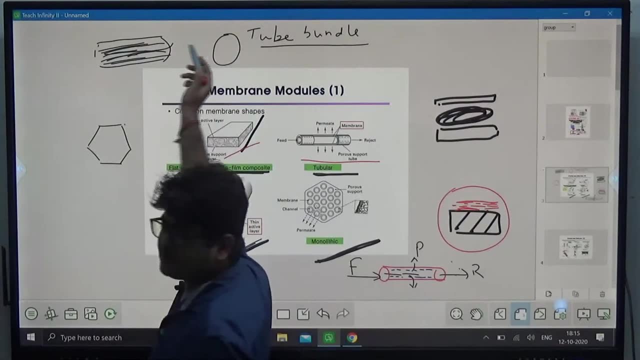 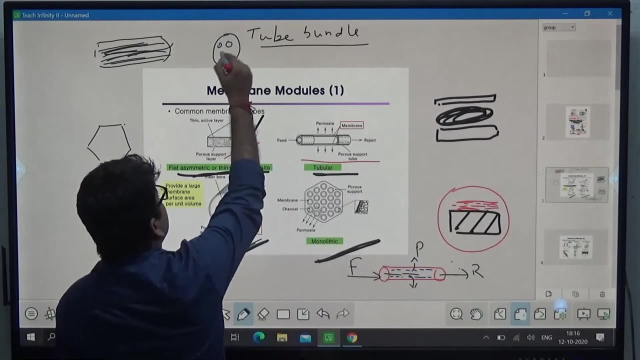 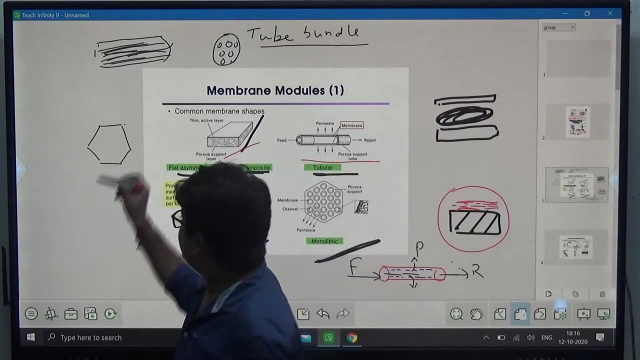 So what happened? these tubes are placed on a bundle, which is called a tube bundle, okay, and we can arrange those tubes based on their pitch, either triangle, in triangular pitch form or in a square pitch form like this, okay, similarly, on a hexagonal, you can say- plate. 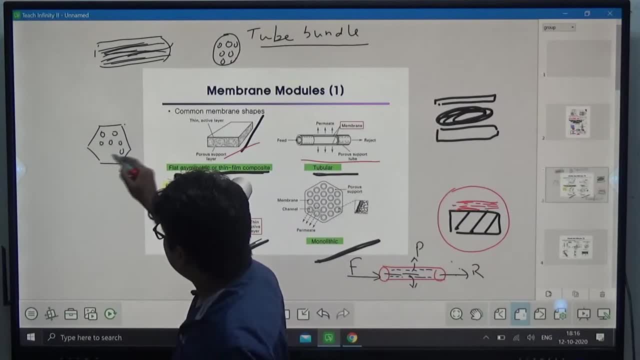 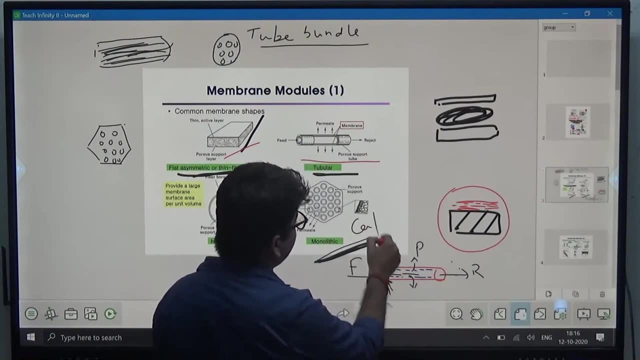 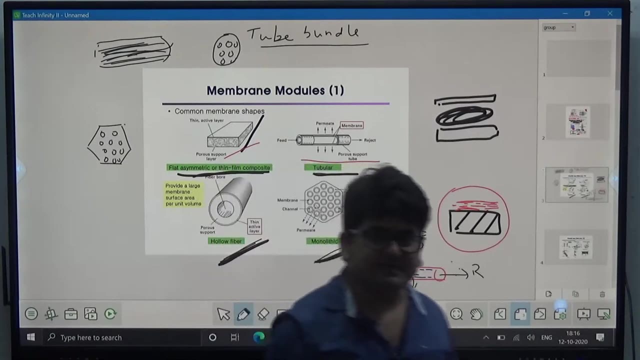 we placed these membranes, Or these monolithic membranes, or you can say kind of a capillary membranes or a capillary tube membranes. all these are same. in detail, we will discuss about them. these are the modules, guys. okay, these are the common geometry of the membrane. if we talk about the industrial 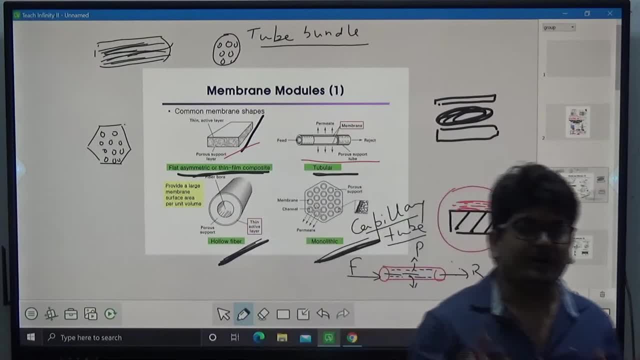 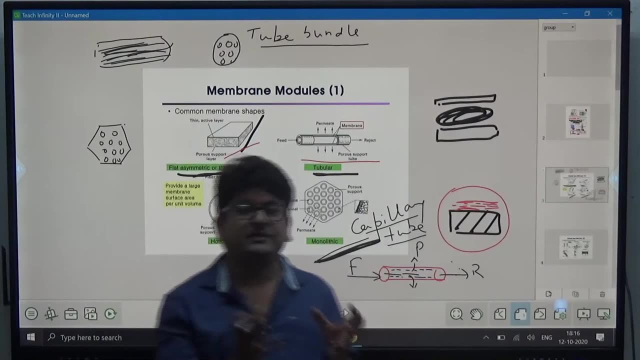 application. Next, if it, I talk about those geometry. how can I place those geometries in an equipment? because membrane separation is one process. So I am going to show you how to do it. So I am going to show you how to do it. 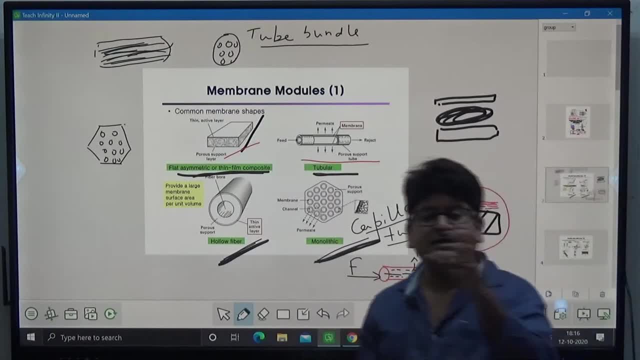 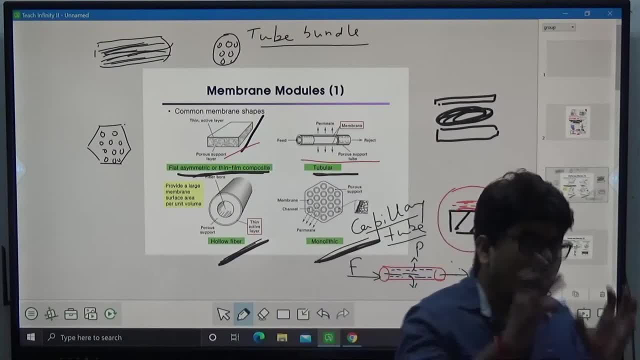 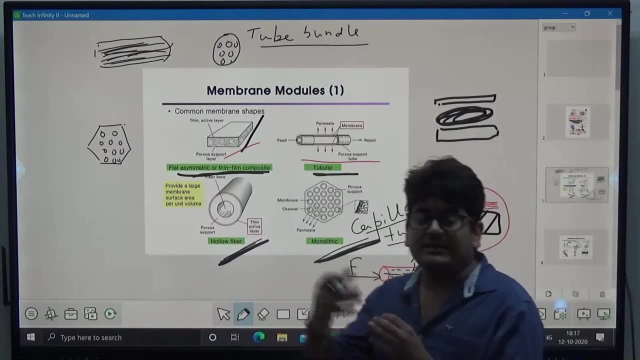 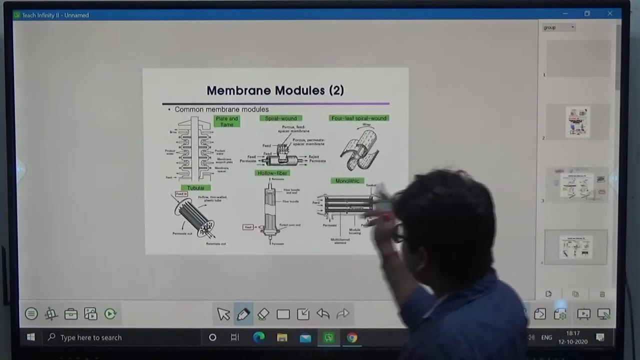 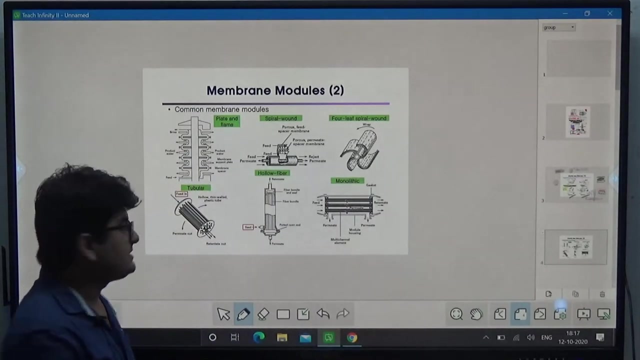 one selected component. okay, So how can we place these membranes, these geometry, these membrane geometry in those equipment which we are going to use for the separation purpose? So for that we have these types of arrangements, these type of equipments, or you can say modules. Those were the geometry of the membranes and these are the modules. 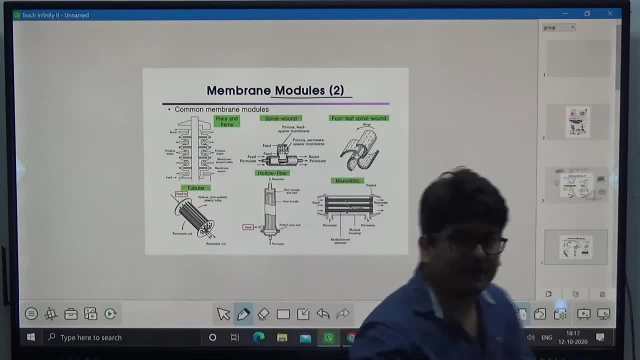 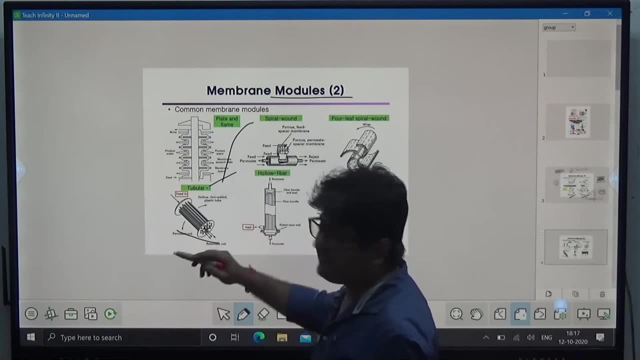 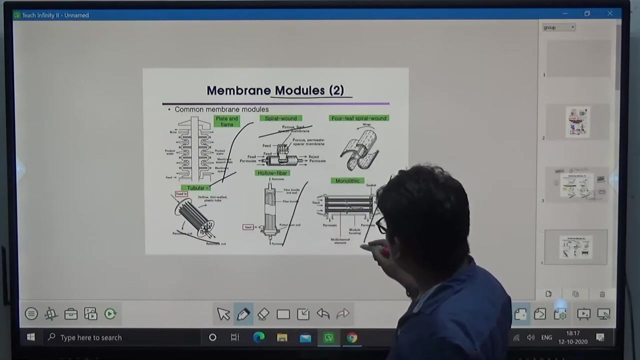 those assemblies in which we are placing the membranes. Okay, one is tubular again. this is the tubular, this is the platen frame filter, this is the spiral bound membrane, this is the hollow fiber membrane and this is monolithic. and this is the four leaf spiral bound. That is a. 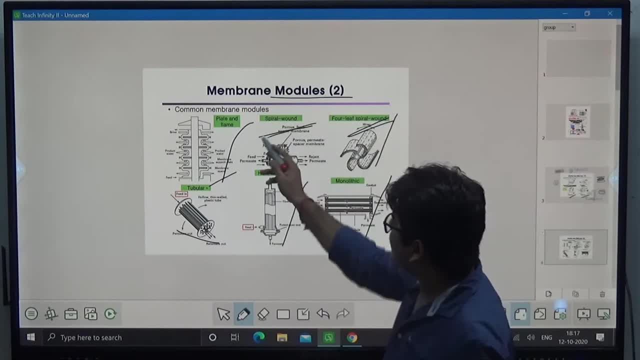 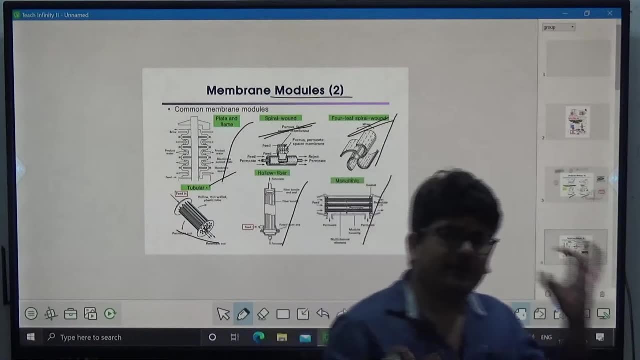 different kind, you can say the modification of a spiral bound membrane. We will not talk about those things as such. We will talk about their working mechanism, how the membrane, the feed is going, how the recontent and permeate we are obtaining. Okay, and then the advantages. 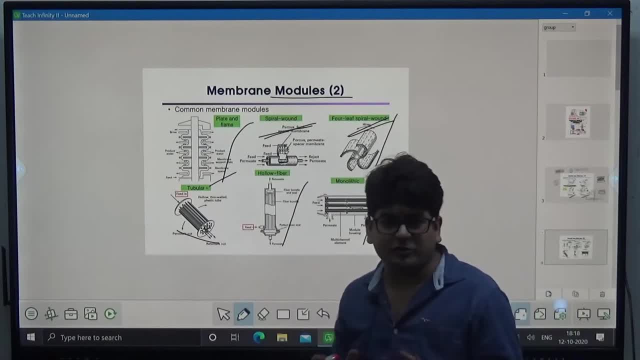 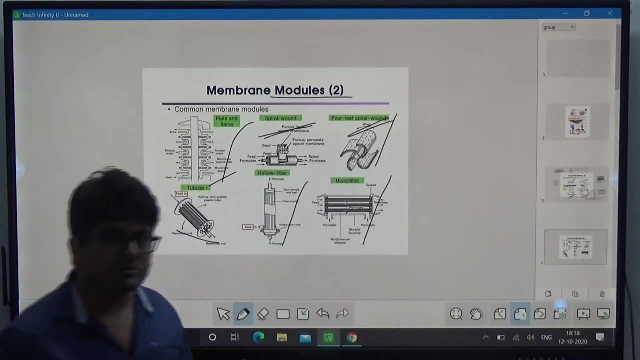 applications and disadvantages of these modules. This is one kind of a theoretical part, But the important thing is the working which we should know, because we don't know in gate exam what they can ask. So we should be ready with all the things. 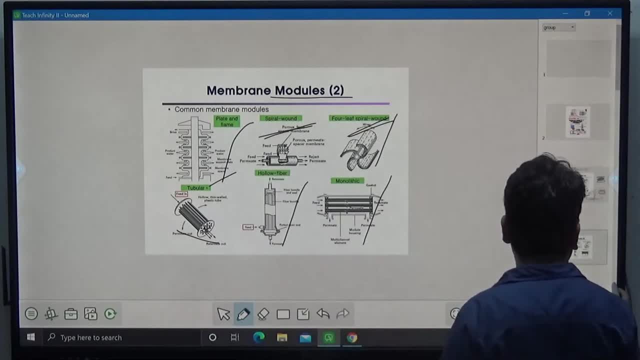 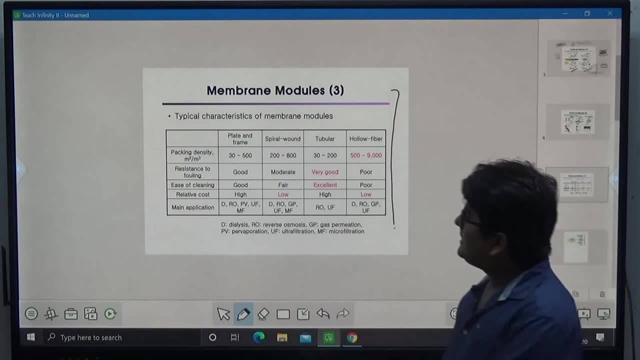 These are the sizes, guys, and the applications of these membrane modules, Okay, and the comparison between all of them, Okay, based on the size, which kind of membrane module we should refer? Okay, so all these things I will provide. I will share the soft copy of this presentation in your 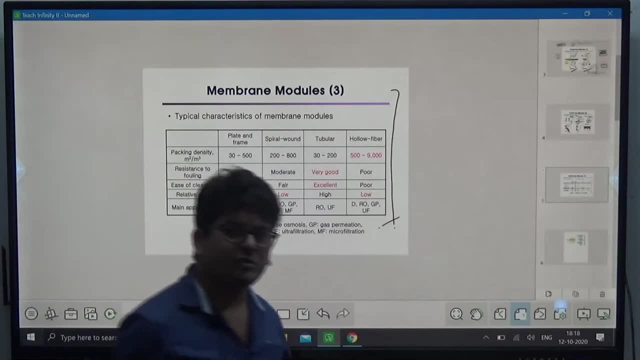 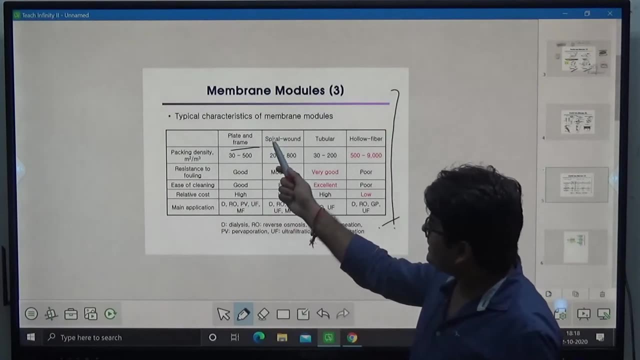 telegram group, You can see all these things. This is the theoretical stuff and we don't need to discuss anything like that. Okay, like in platen frame membrane modules, the packing density is 30 to 500 meter square per meter cube, where meter square is the membrane area. membrane separation. 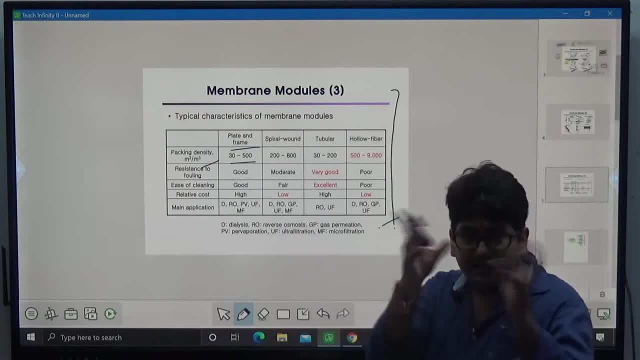 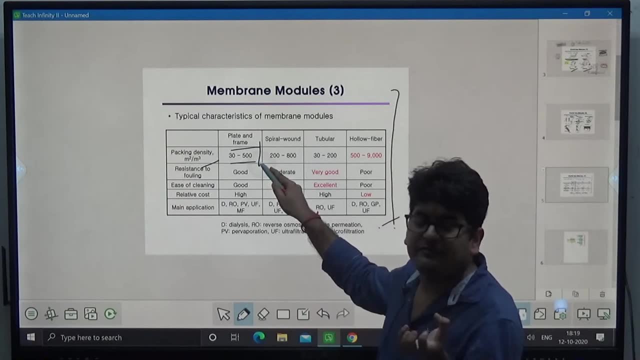 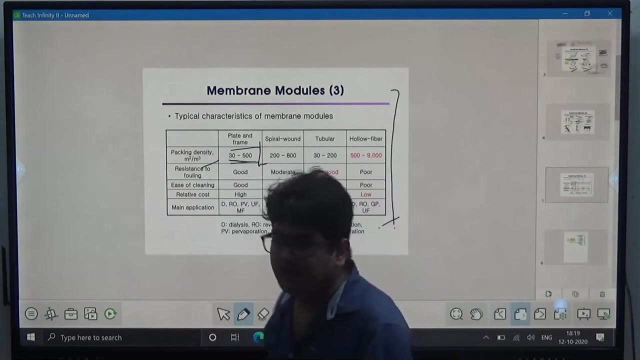 area of the membrane and meter cube is the volume of the assembly. Okay means in one meter cube of platen frame module the packing density is 30 to 500 meter square. per meter cube, where meter square is the ene module platen frame assembly, we can have 32, 500 meter square of membrane area And that is. 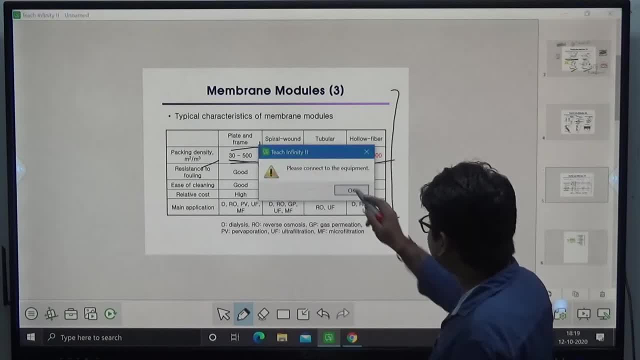 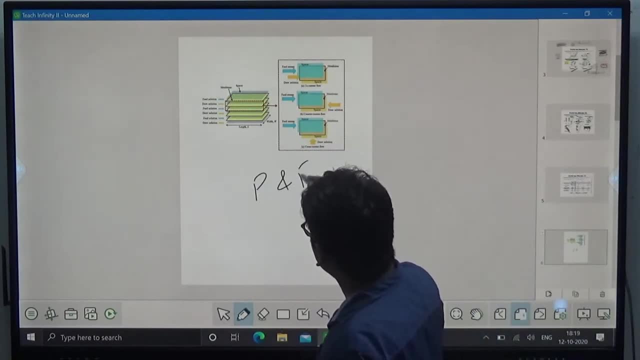 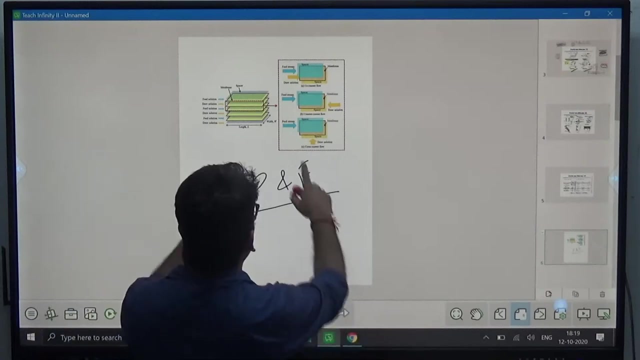 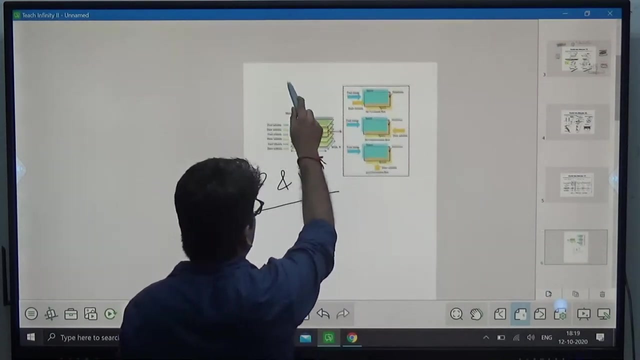 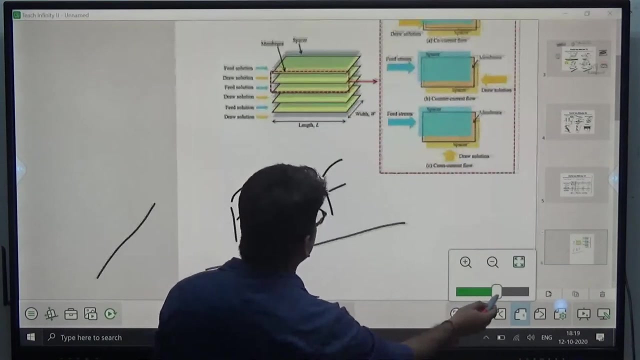 largest in the Holo fiber membrane modules. Let's talk about the working. This is, guys: platen frame modules- closed, absent flatels and membrane modules. what happened? as you can see, I am not comfortable with this part as such. still, yes, this is the function. okay, correct. 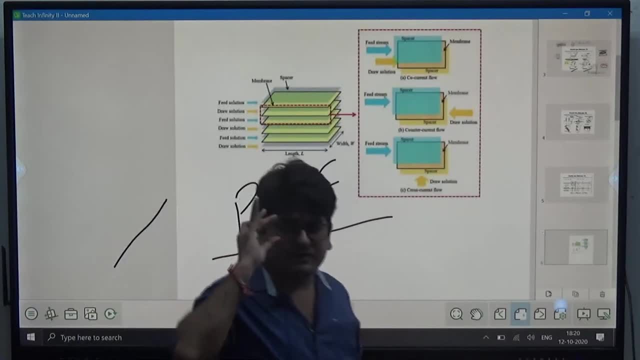 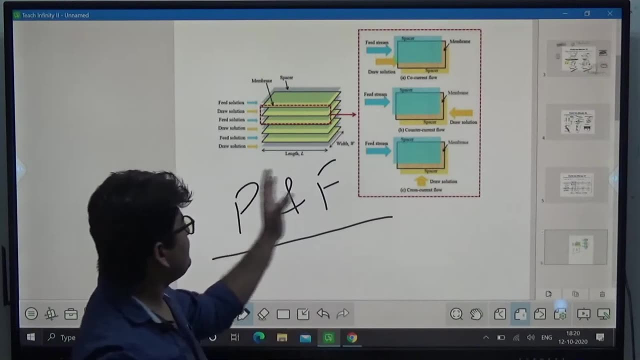 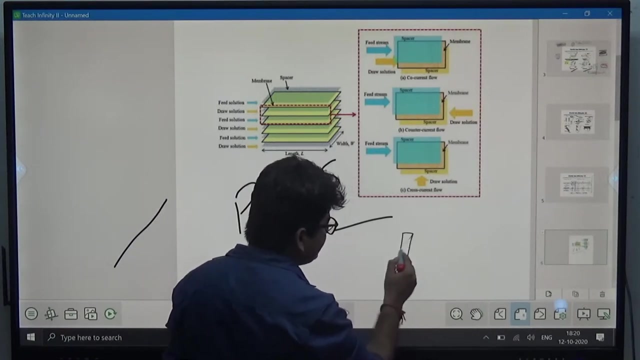 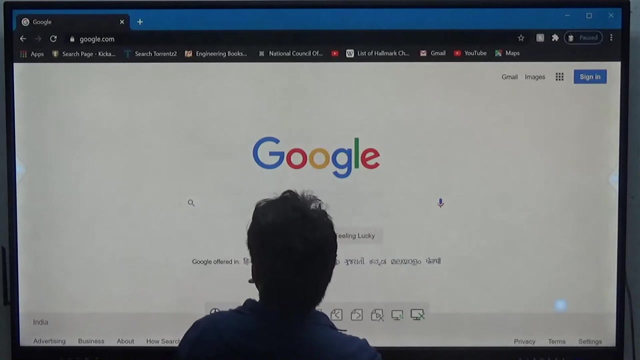 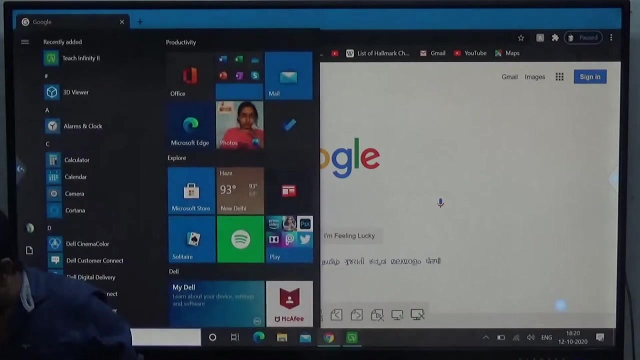 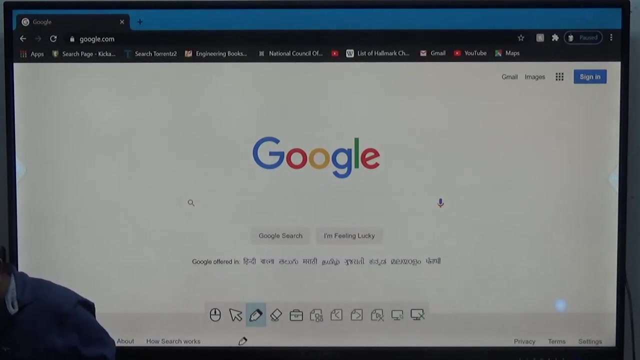 Okay, what is happening here? See, if you have heard about the plate and frame filter traps in filtration in mechanical operations, just like that, this is a plate and frame membrane module. What happened? We have one plate- you can say one solid plate and one. where did it go? come on, brother. 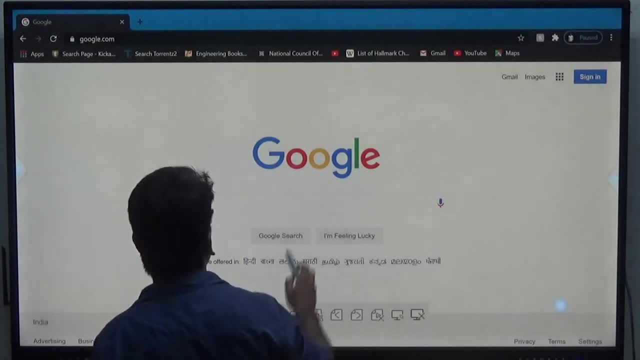 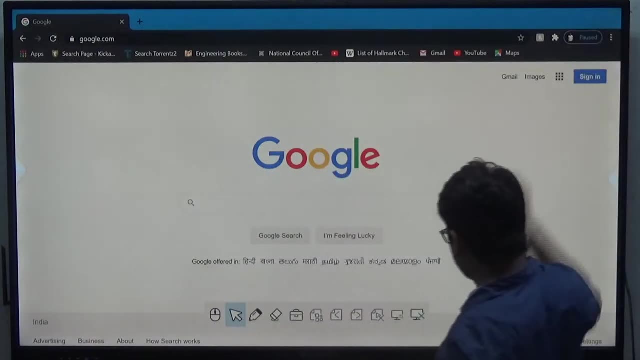 I have to say: one solid plate. where did it go? The one at the top? there it goes. there it goes. okay, there it goes. We have one plate. here's a surface layer. What happened? See that now. 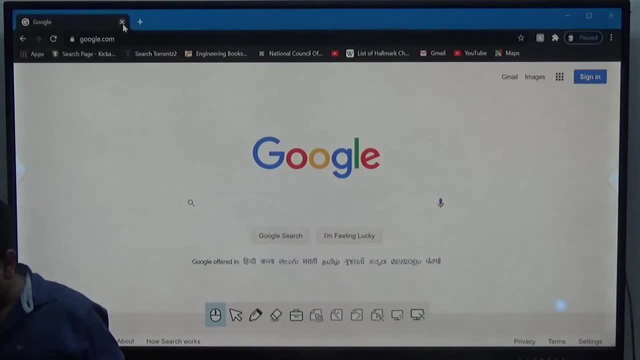 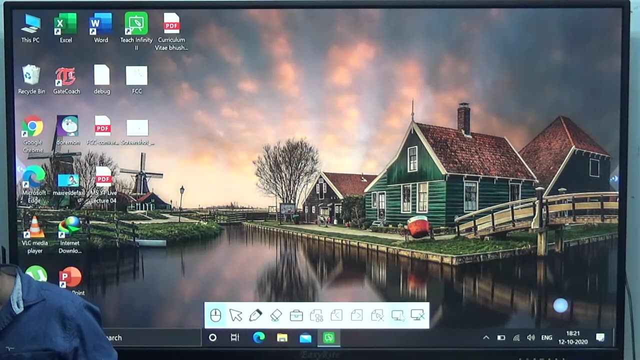 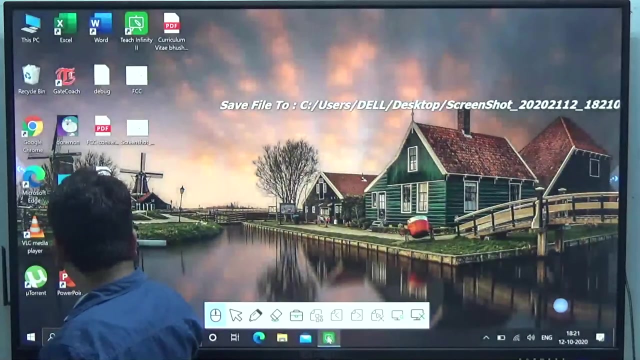 So what has changed? I mean, what has changed is that we have a plate where we can see where the campaign was, So you can see some of it. Good, All right, Just a minute, guys. let me get back to the file. 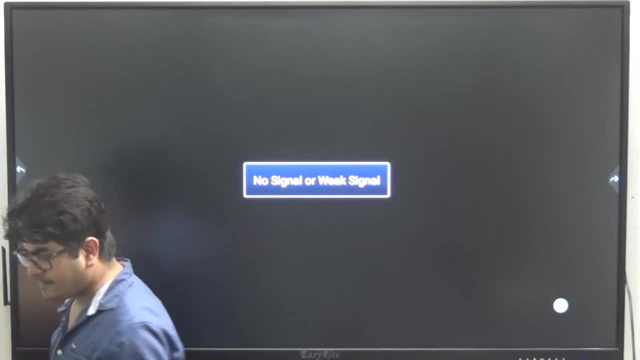 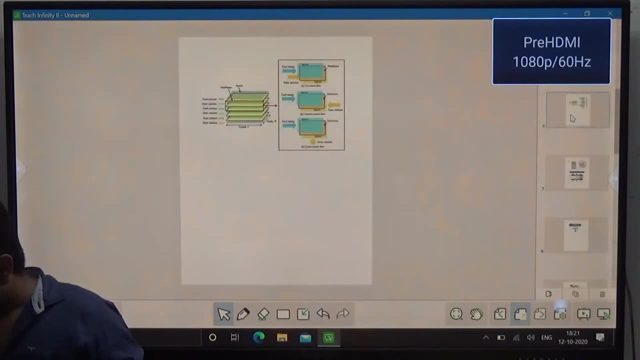 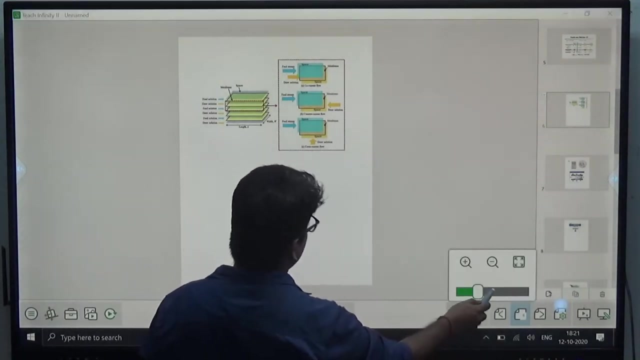 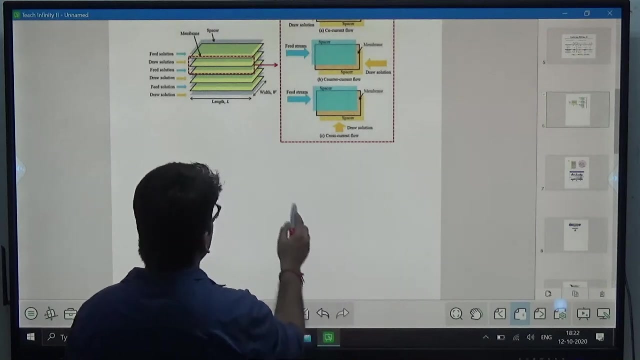 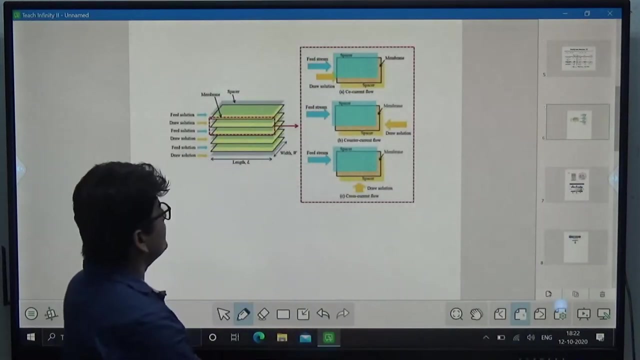 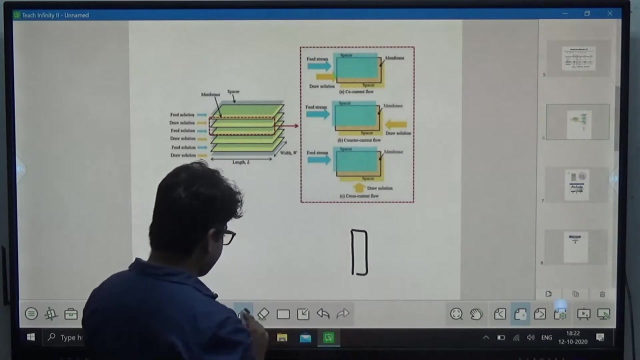 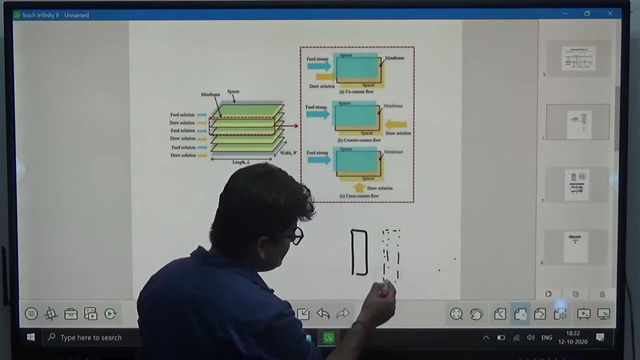 Thank you. So what happened in plate and frame module? see, we have one solid plate and one hollow fiber hollow frame. you can say in which our membrane is present, the membrane material is present, like this, in that frame. or you can say: this entire frame is actually a membrane. 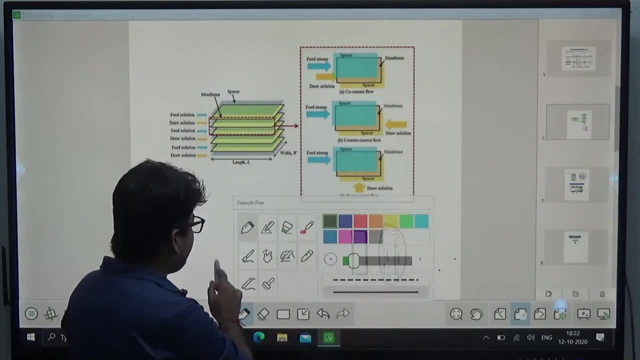 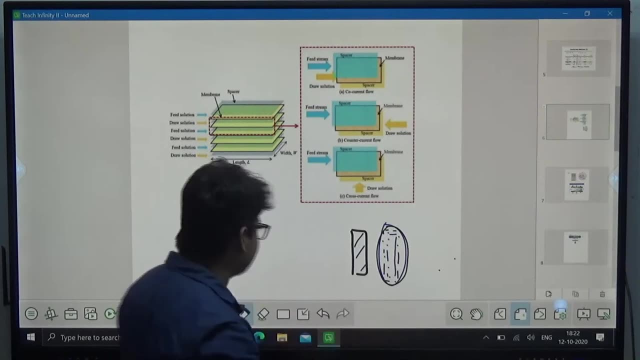 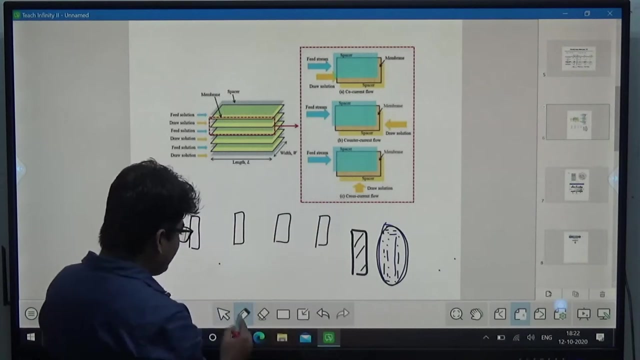 Okay, So we place these membranes and frames, these solid plates and the membranes in alternative arrangement, like one plate, second plate, third plate, fourth plate, and in between them we have placed our membranes like this: This orientation can be vertical, this orientation can be horizontal, like this or like this: 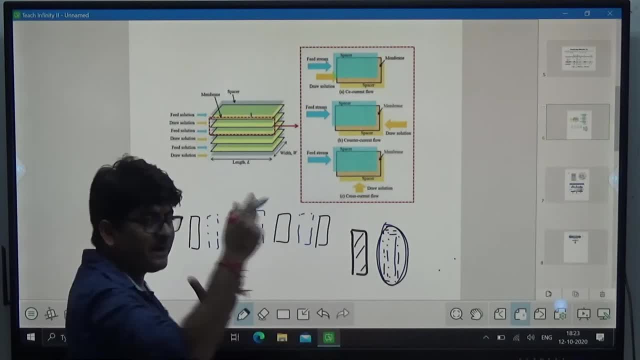 This is the vertical orientation, where we have placed the membranes in a vertical formation, in a stack formation, one on top of each other. So here what happened: we send the feed in this, these plates where the feed enters in this. 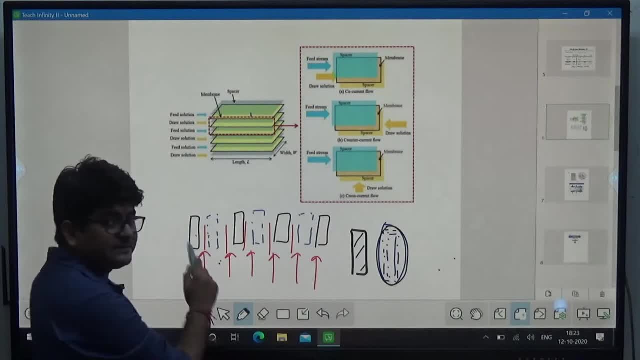 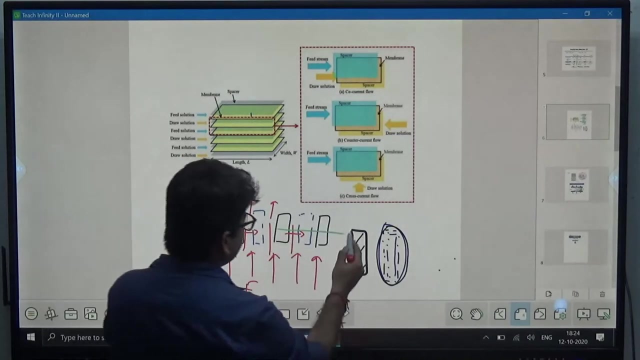 Okay, Okay. So the feed comes in contact with these membranes, So permeate will go inside the membranes and here we will get the residual part. Okay, Or you can say retentate and this entire permeate, this entire permeate, we get through the frames. 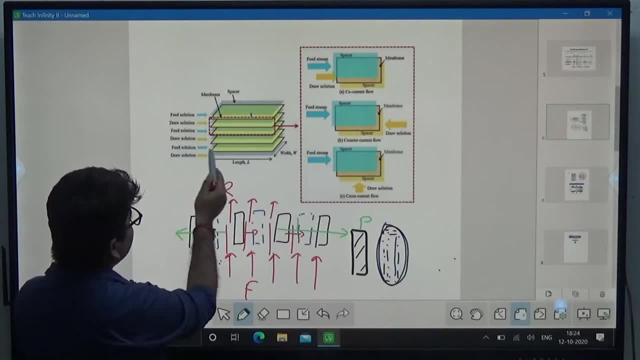 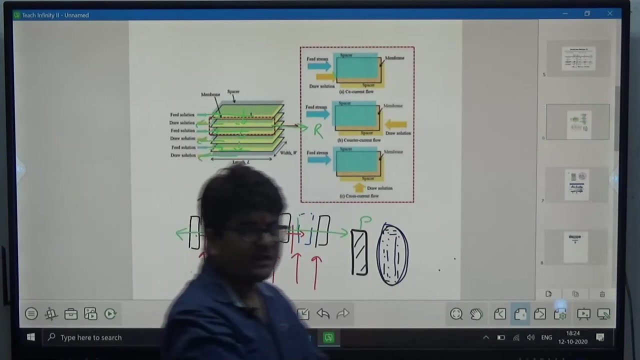 on the other side. Okay, So you can see. we are sending the feed in between these plates and frames. As feed enters in this, the permeate will cross the boundaries and here we will get the retentate and the solution, the retentate solution. we will get back in the opposite. 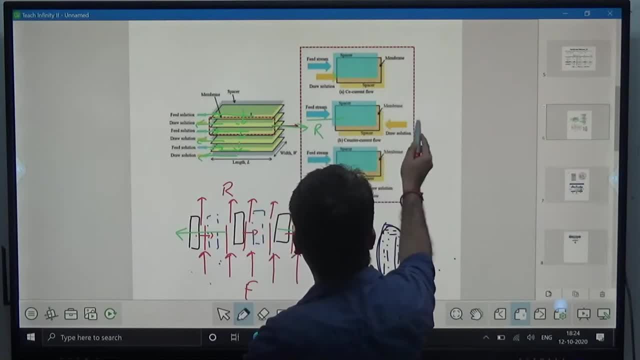 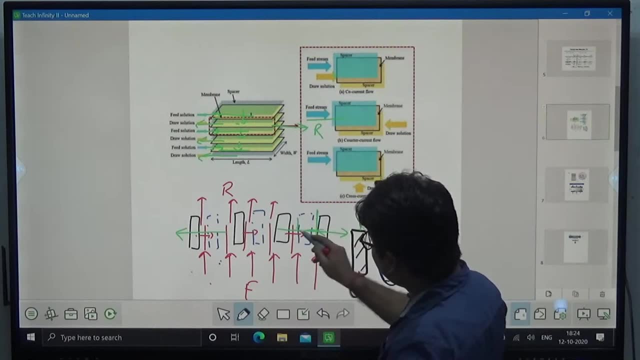 direction. Okay, This is the. that's how they work. Feed enters in between these plate and frames, permeate crosses the membranes and here we get the retentate and the permeate. we get back on the other side of the column. 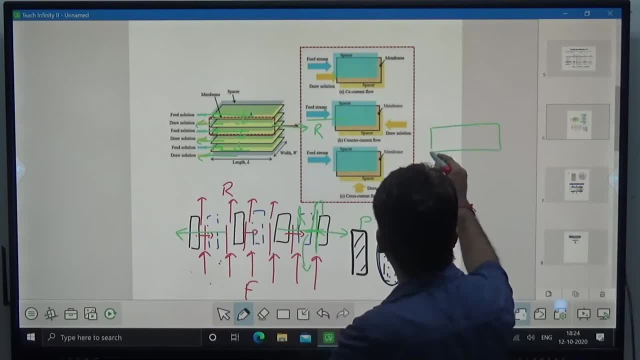 Like, if you want to draw the equipment, you can draw like this: Okay, This is the, these are the plates. Say: this is the solid plate, then a frame. a solid plate and a frame. a solid plate and a frame. 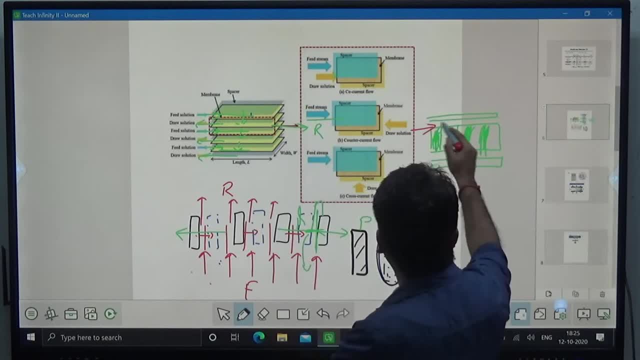 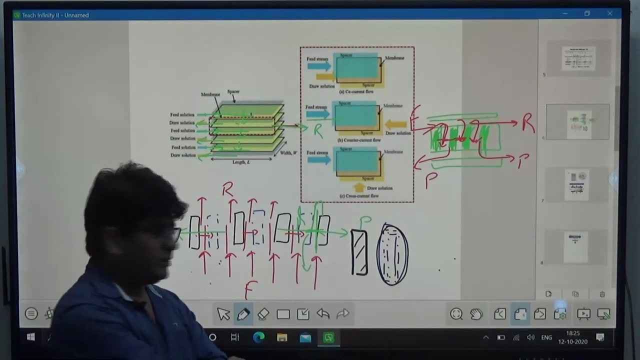 We send the feed in this it crosses, it enters in these frames, permeate crosses the membranes and here we are supposed to get the retentate and here in the bottom we get the permeate. Okay, That is the working of plate and frame membrane modules. 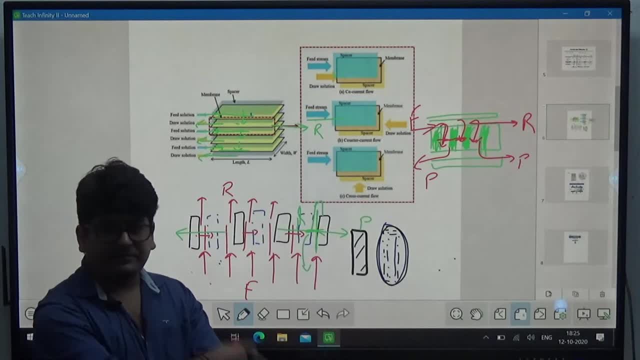 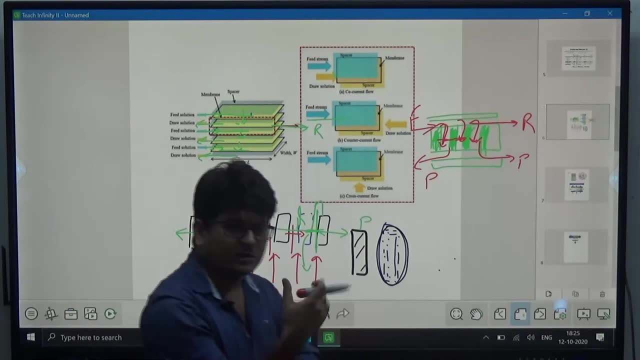 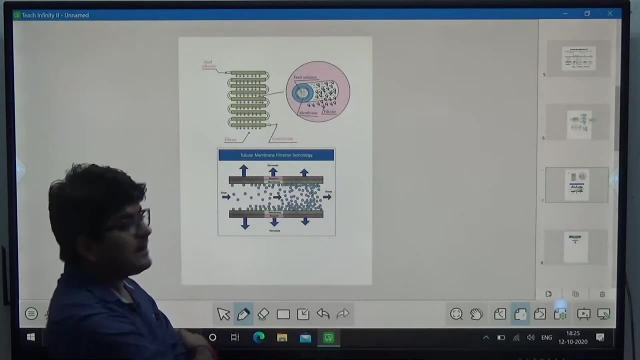 And the direction of the feed and the permeate we are obtaining. based on that operation, we can classify the flow as counter current flow, co-current flow or the cross flow. We will discuss that thing as well later on. The next is the tubular membrane. 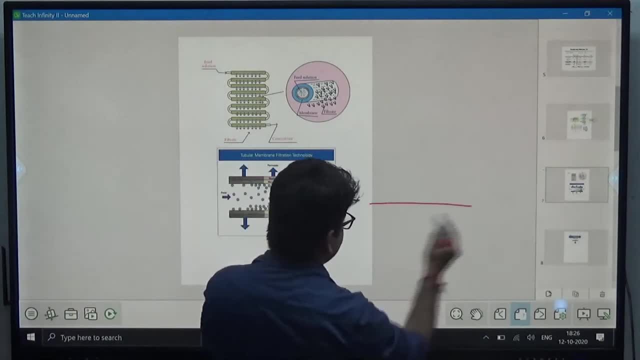 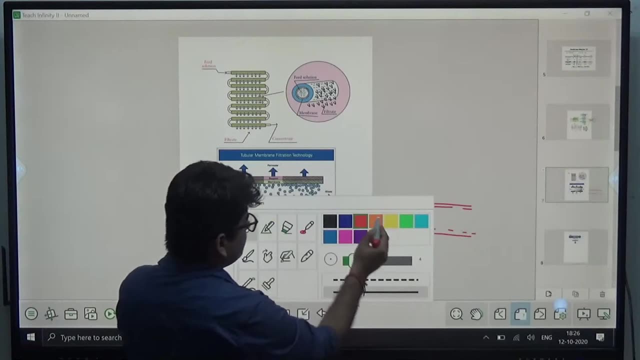 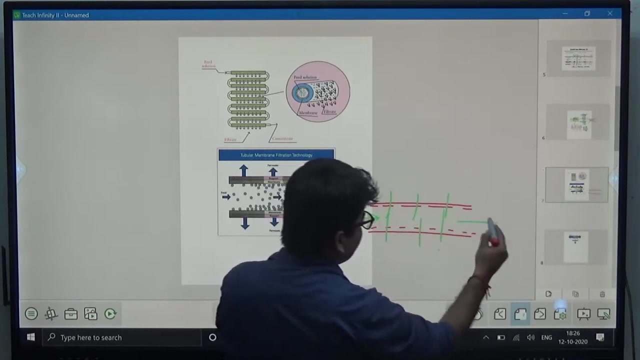 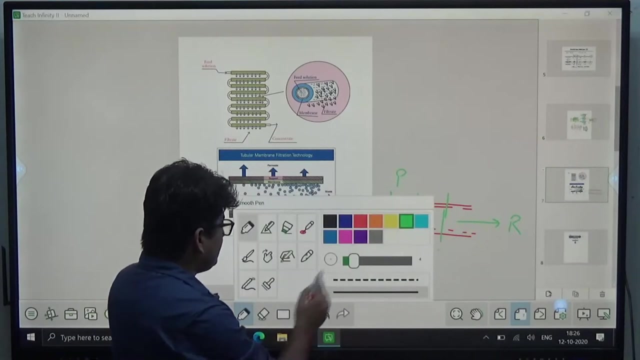 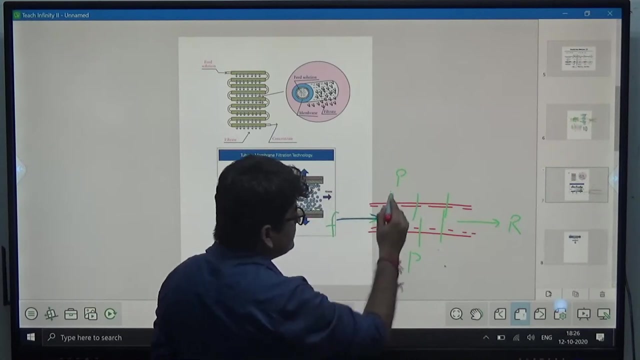 As I told you, we have a pipe In which we place these membranes. We send the feed, permeate crosses and here we are supposed to get the retentate. So here one thing is very important to understand: Okay, As feed enters in the pipe, you can see permeate is crossing the membrane. 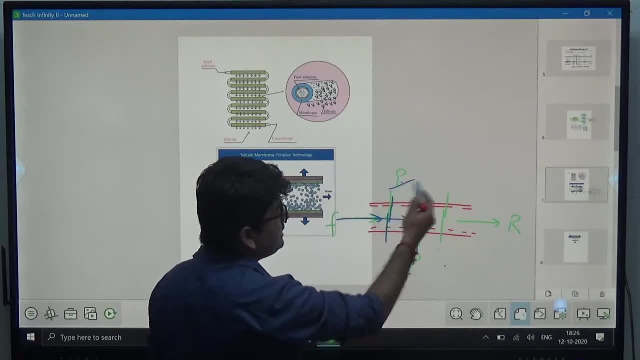 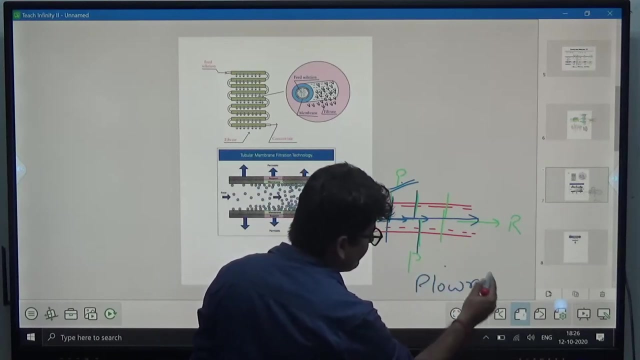 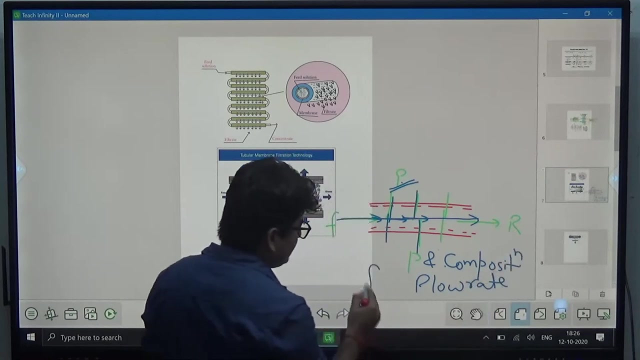 The membranes And we are obtaining the permeate on the other side. Okay, And here you can see as this feed moves further, as this feed moves further along the length of the pipe, the flow rate and the composition. the flow rate of the feed and the composition. 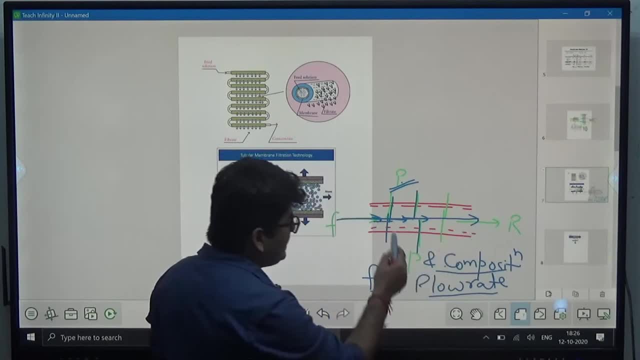 of the feed will change Means at any time, Means at each and every point inside the pipe at different length. if you consider this point, this point, this point or this point, the feed rate and the composition will be different because simultaneously the permeate is separating. 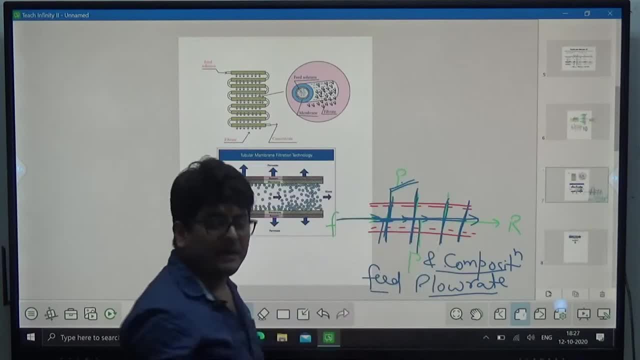 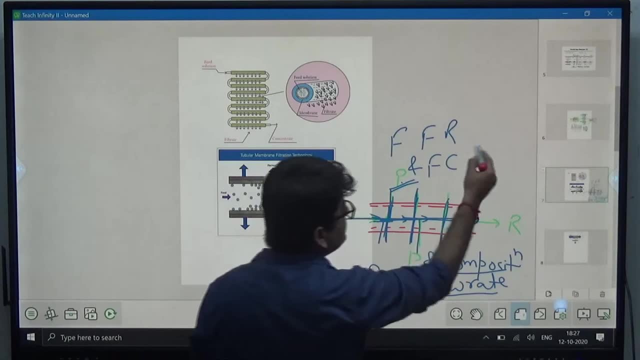 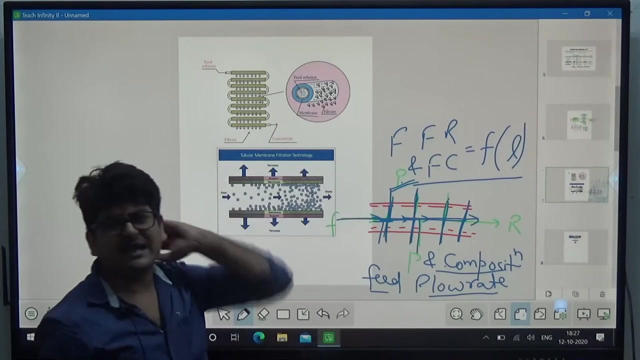 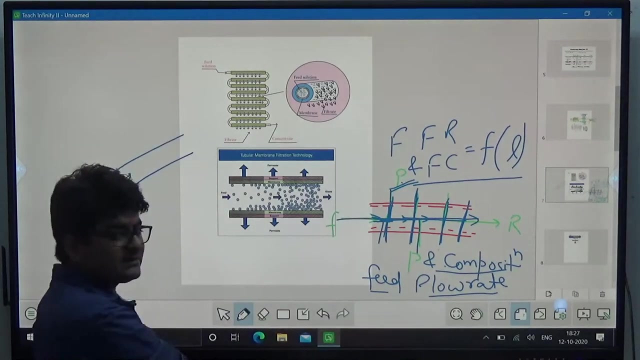 Okay, So here, in case of tubular membranes, we can say that the feed flow rate and the feed composition is the function of length, Length of the tube, just like the plug flow reactor. In case of plug flow reactor, if you remember, as feed enters along the length concentration. 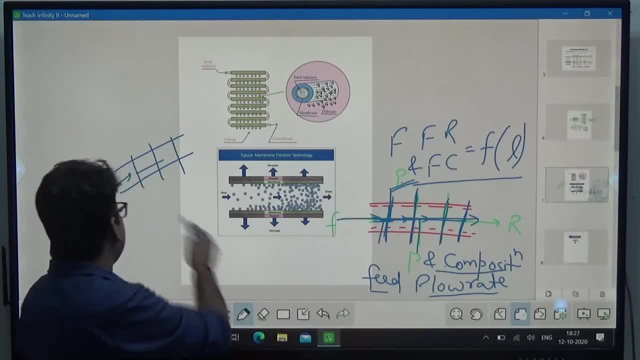 changes because reaction is taking place. So we say that concentration is the function of length. Similarly, here the flow rate and the composition of feed will be the function of length. And what will be the composition? if I ask you the feed composition, it will increase. 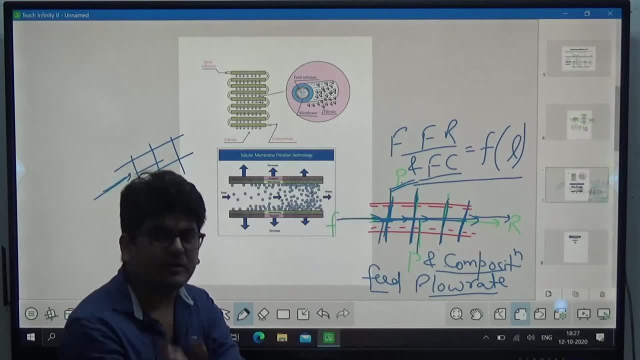 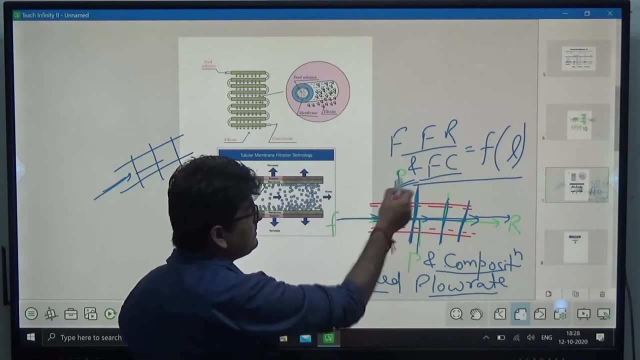 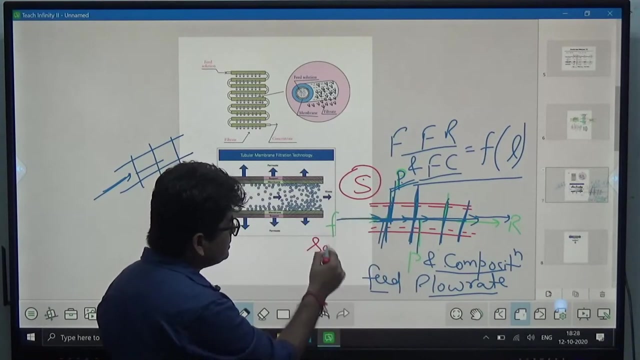 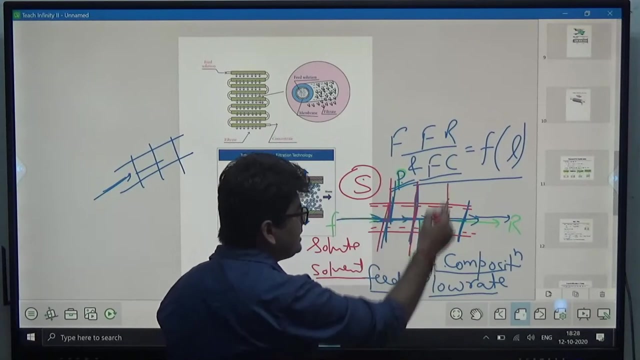 or decrease. Basically, the feed will get concentrated or diluted. What will you say If the solvent is separating, if the permeate means, if the permeate means solvent? suppose feed has solute and solvent. Okay, So solvent molecules are moving through these membranes. 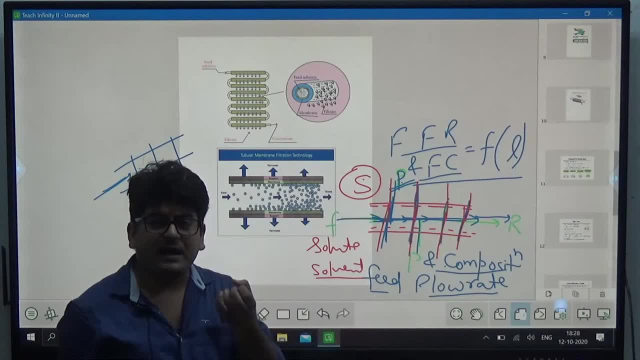 So you can see that along the length the solvent amount of solvent will decrease. So ultimately the concentration of the retentate will be higher than the concentration of feed. So this is the tubular membrane module. Here we send the feed permeate passes through these surfaces from the outer surface of the 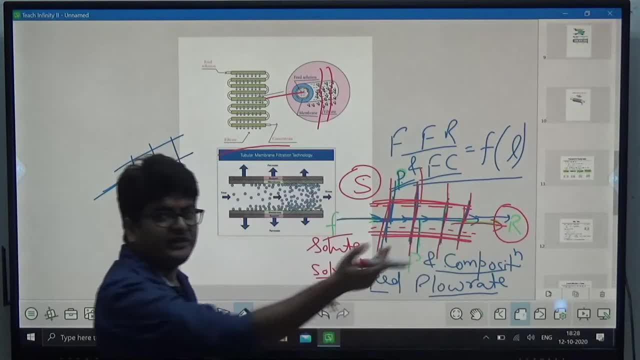 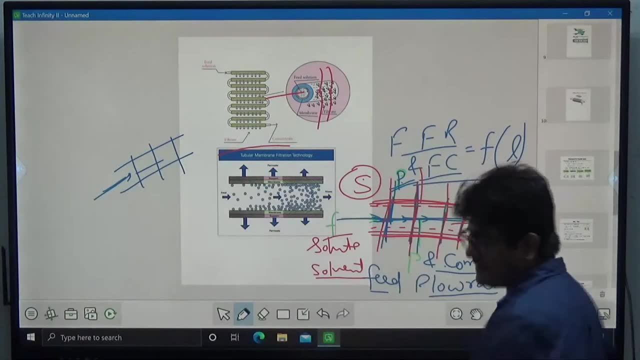 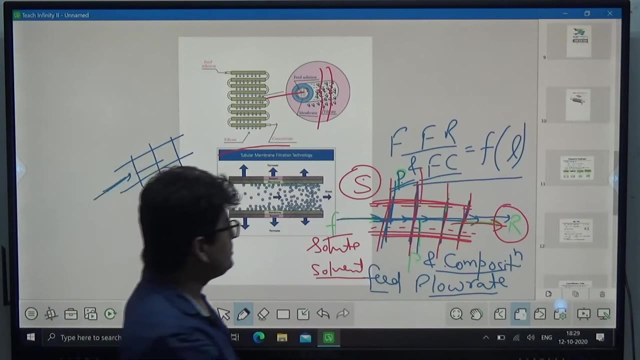 tube permeate passes and on the other side of the tube we get the retentate. This is the working of tubular membrane module. I hope this is clear guys. Yes, I told you. the PPT we will share in the telegram. 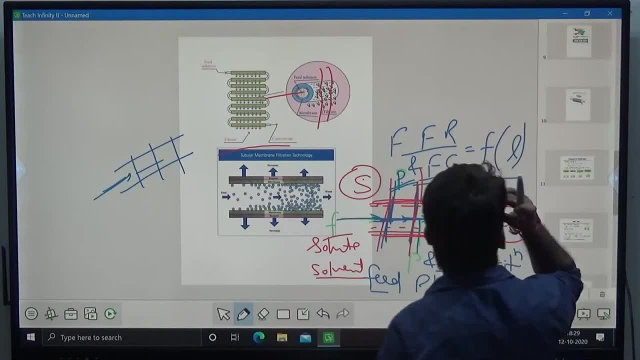 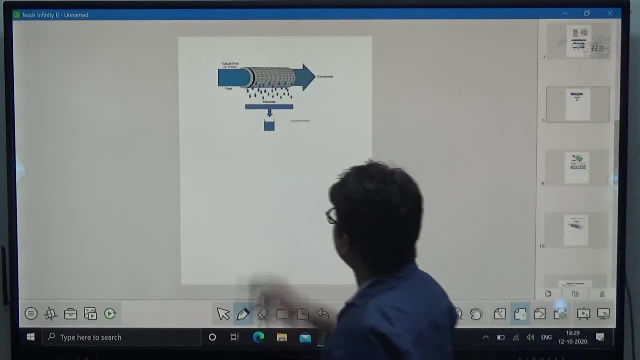 So you can download that there. Next is the tubular membrane. You can see Feed is going through the outer surface. We are getting the permeate And here I am getting the retentate. Okay, So you can see that retentate is more concentrated than the feed because solvent molecules are. 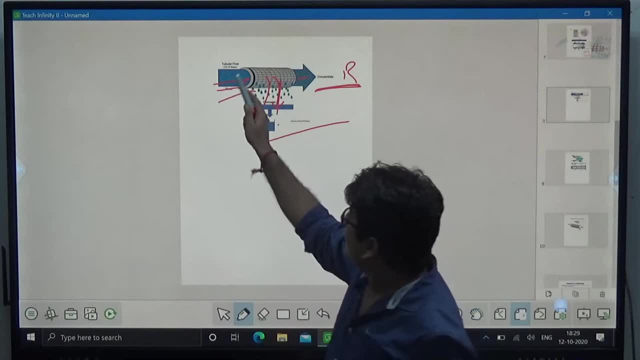 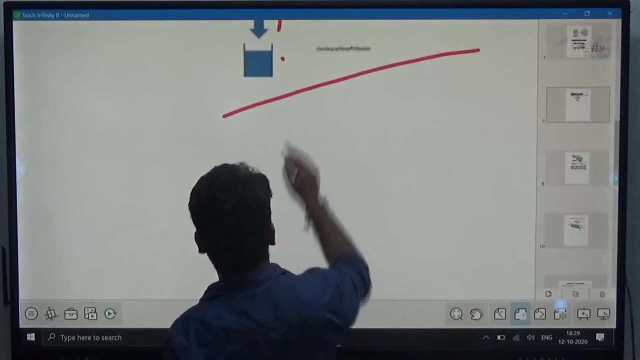 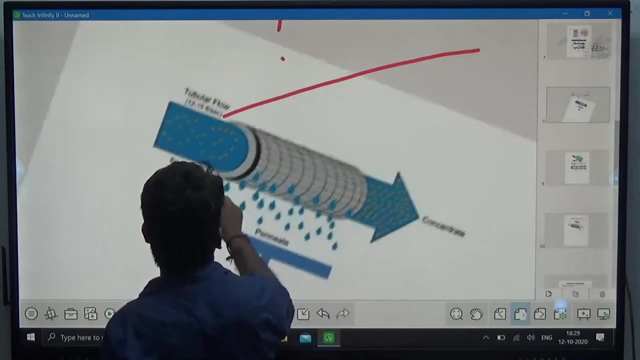 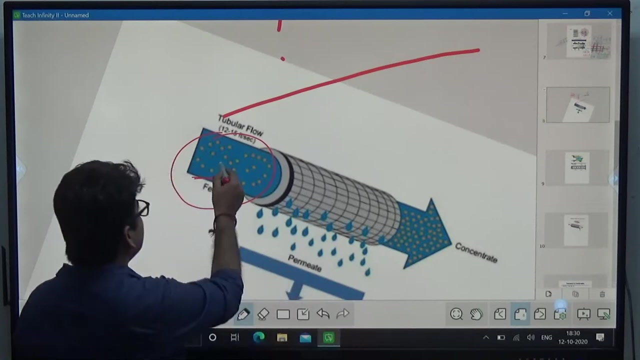 leaving. This is the solvent. You can see water And these are the solute molecules. Okay, I hope Here you can see. This is the solution, where this liquid part is representing the solvent and these dot dots are the solutes. 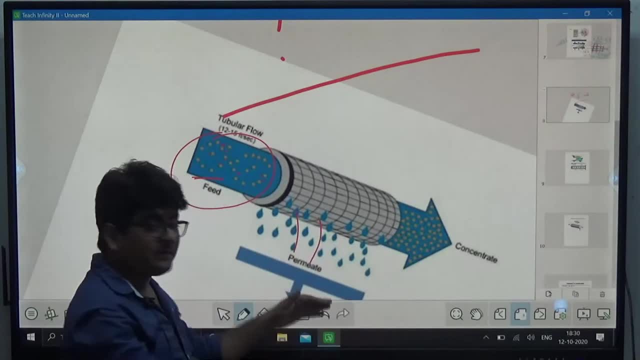 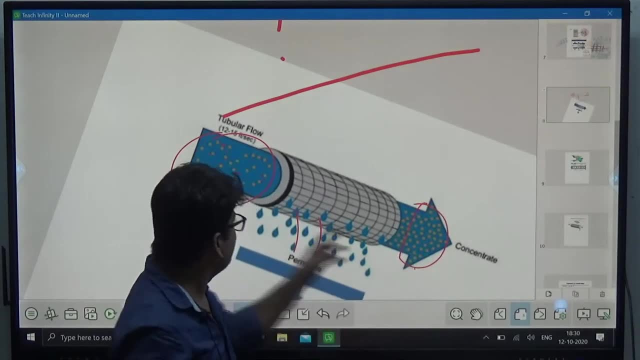 Here only solvent is crossing the permeate. Solvent is coming as a permeate, So here the amount of solute will remain same. Amount of solute will be same, but amount of solvent will be less. That's why the concentration will be higher. 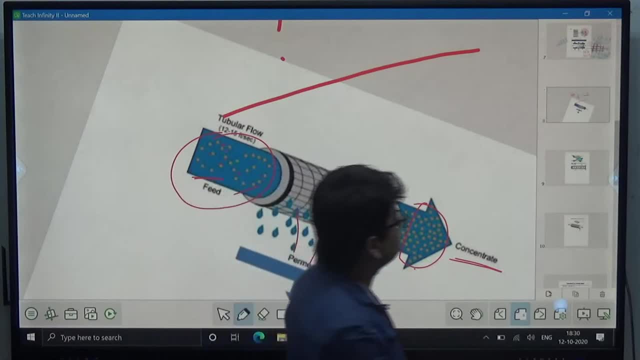 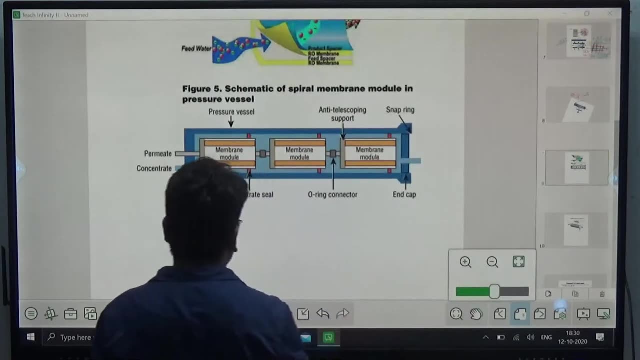 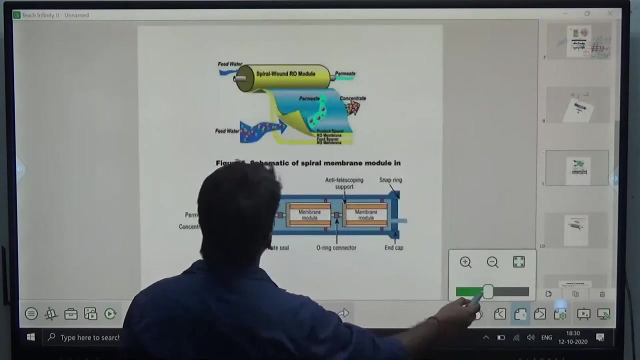 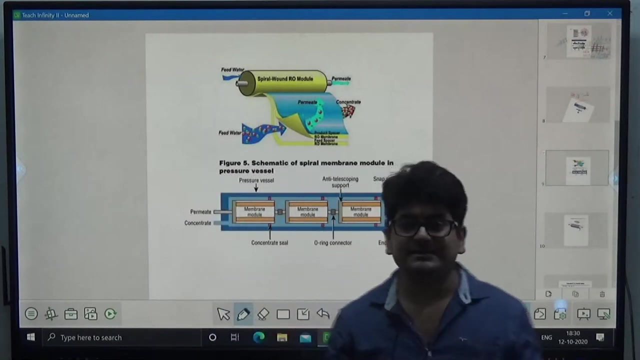 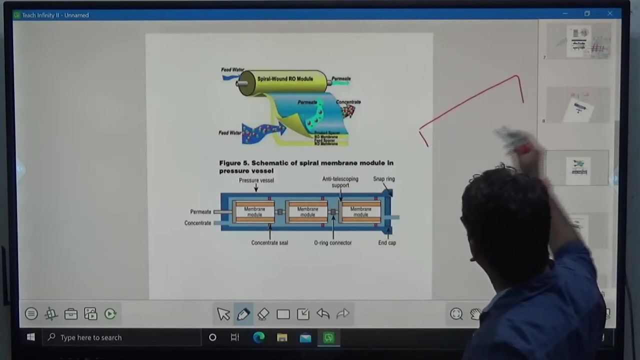 Okay, So this is the working of tubular membrane module. Next is the spiral bound membrane. So what happened in spiral bound membrane? You can consider that just like a bed sheet, We have bed sheet. You know bed sheet. Bed sheet is a long vertical thin layer of cloth threads combined together. 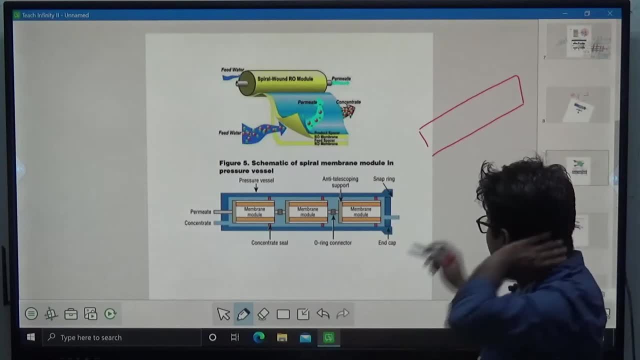 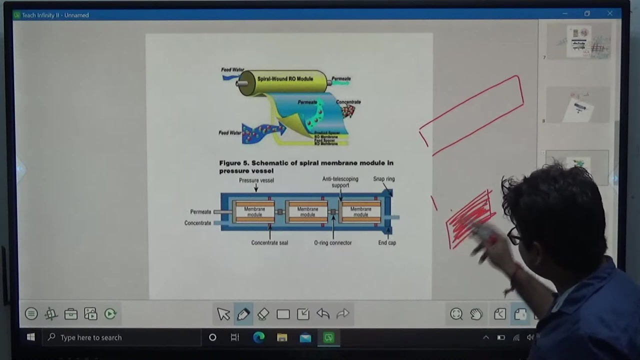 Okay. So here what we can do. If you consider a plate, How can I draw a plate Like this? If I draw a plate, This is one plate. Or you can say one bed sheet. Okay, This is one bed sheet. 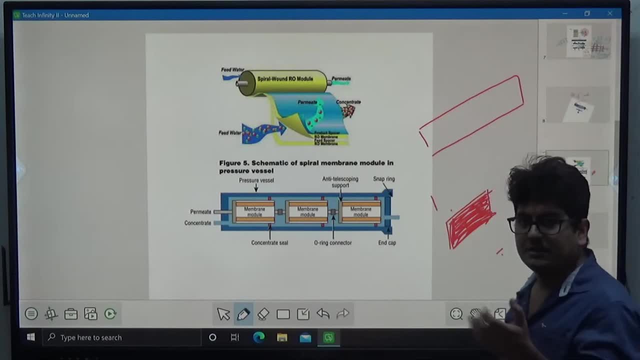 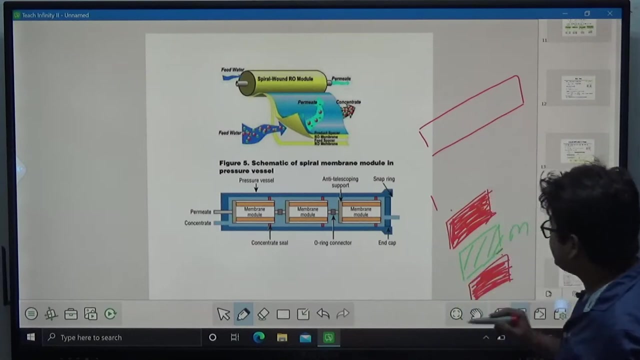 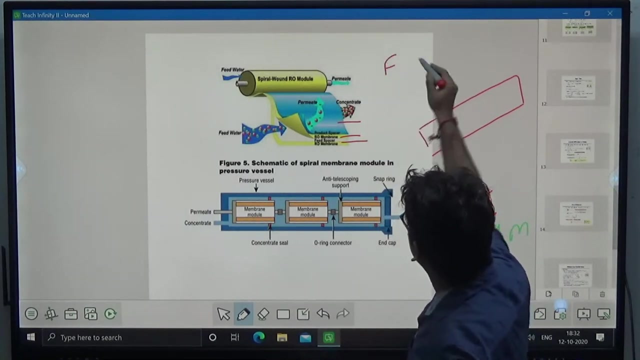 Just above this bed sheet, I placed a membrane. I will place a membrane, Okay, And again there is a bed sheet. So membrane is placed between two bed sheets. you can consider: we have a membrane that is placed between two bed sheets like this: sheet, membrane, sheet, fiber. this is the 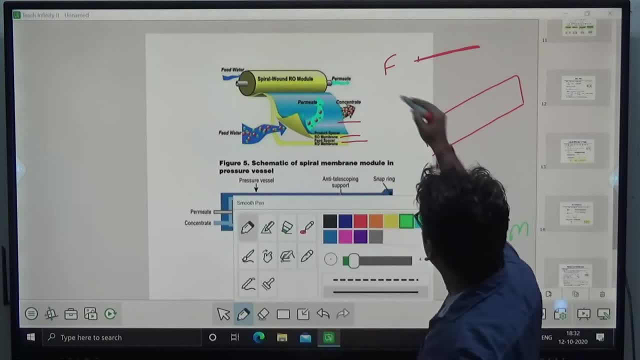 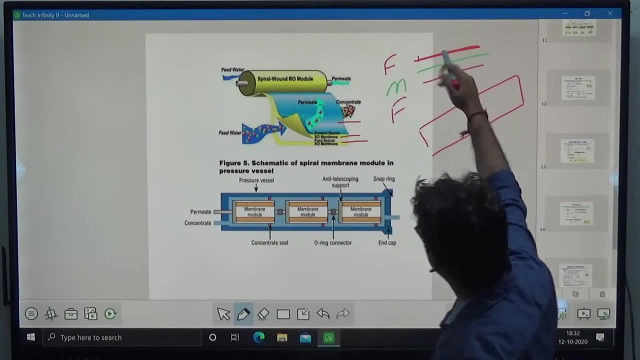 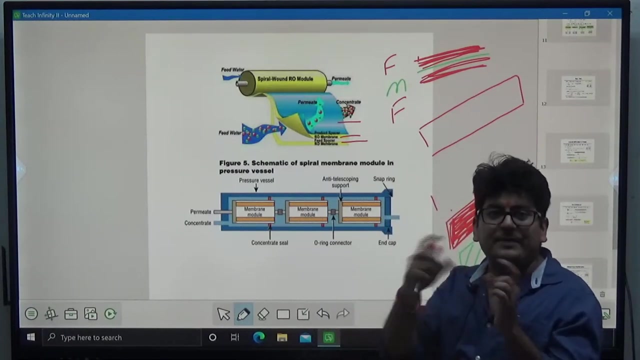 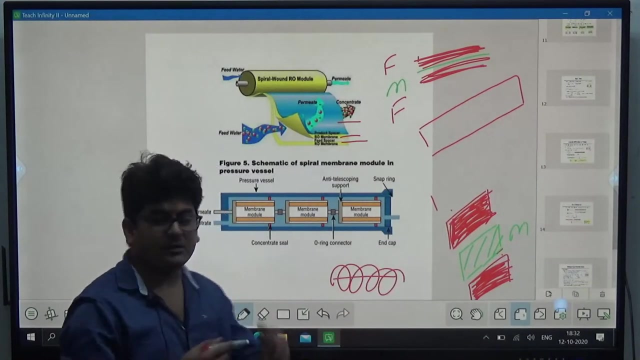 fiber. this is the membrane and again, this is the fiber you can see. so, just like when you, this is one bed sheet. so when you put that bed sheet on a pipe, suppose we have a roll and you roll that bed sheet like this: okay, we make a roll of that bed sheet. I. 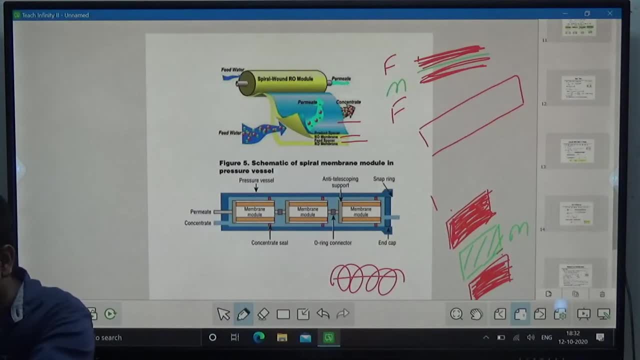 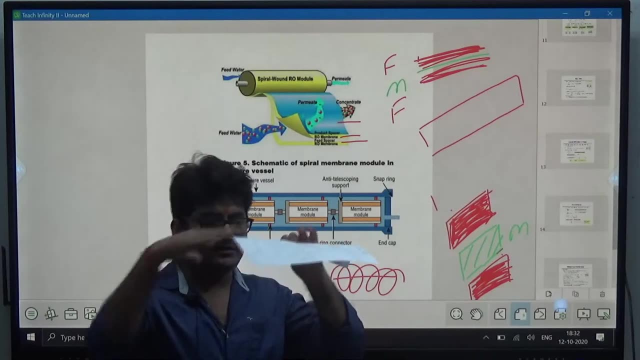 can say, like, if you assume, Okay This, if you consider this is a sheet in which bed sheet membrane and bed fiber membrane and bed sheet is there. now what I am doing, I am making a roll of this, okay. 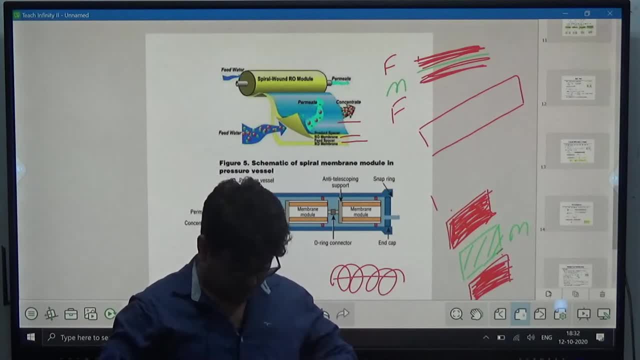 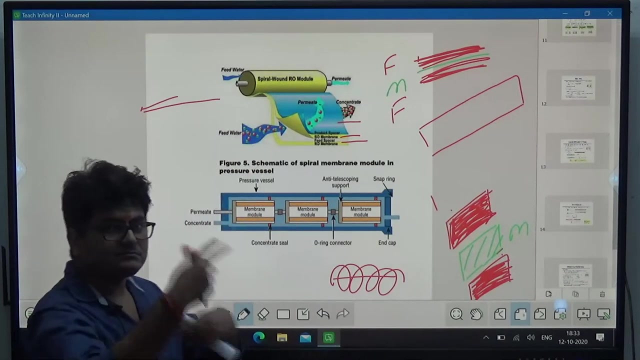 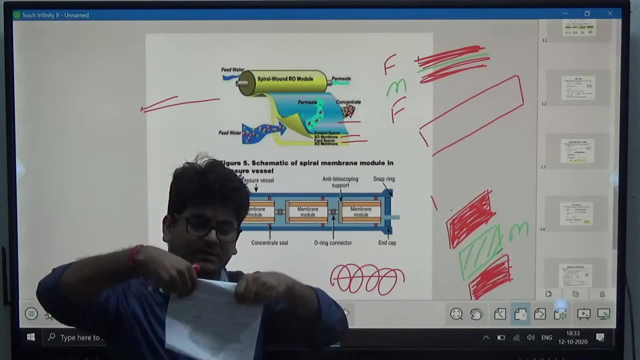 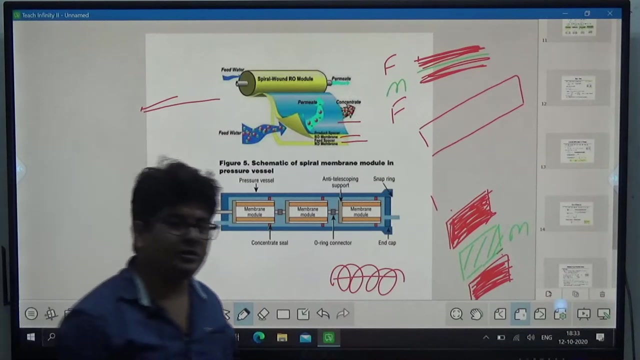 If you have seen any person like this- a roll, a spiral bound- okay, I have made one spiral bound. This is a pipe on which I have just rolled down that thing on each other. okay, That is the spiral bound membrane. simple spiral bound membrane module. 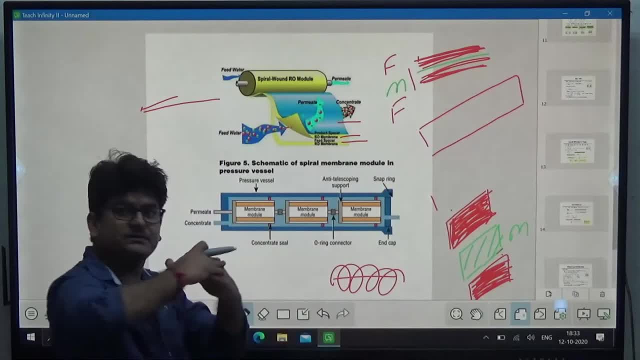 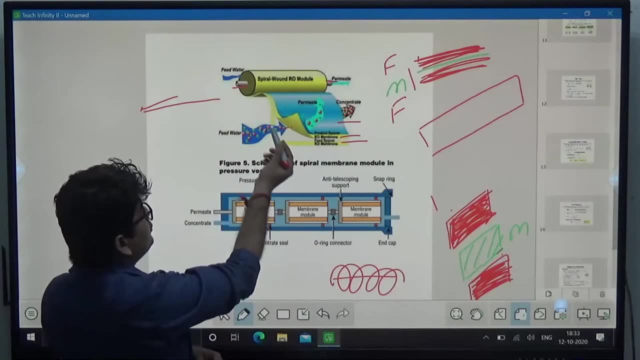 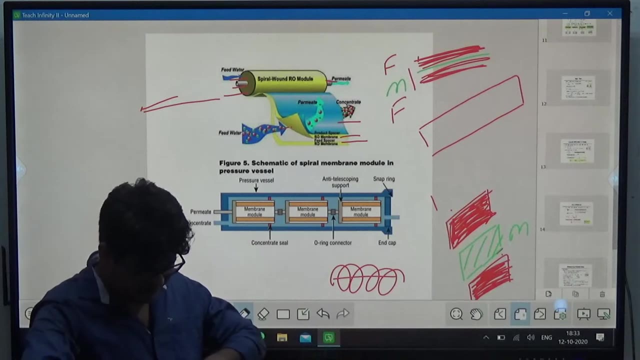 This is the sheet having these three things and I have rolled down that sheet on each like this on a pipe: Okay, Okay, So what do I do In that, between these rolls like this, if I consider? try to explain this to you. 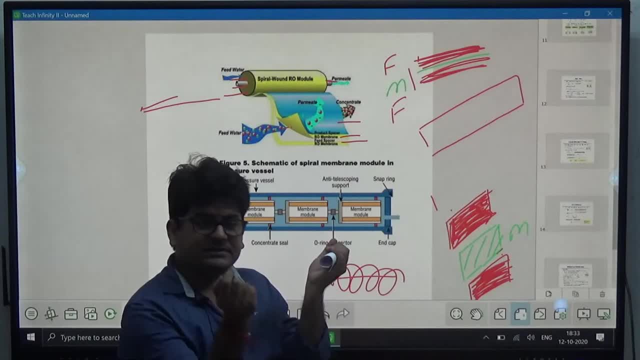 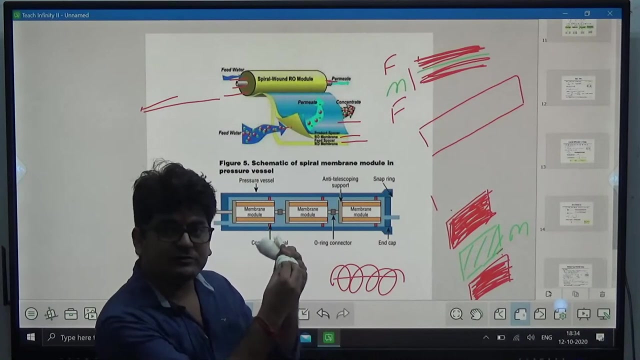 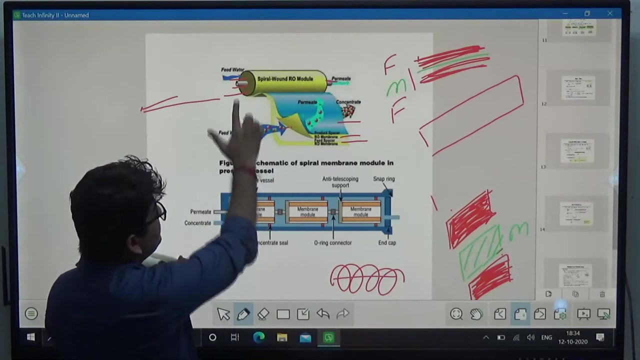 I have made this roll. okay, Now send the. this is the roll. Now what I have done: I am sending the feed inside this. in between these bounds, all these layers, I am sending the feed. feed will enter in this. okay, feed will enter in this. 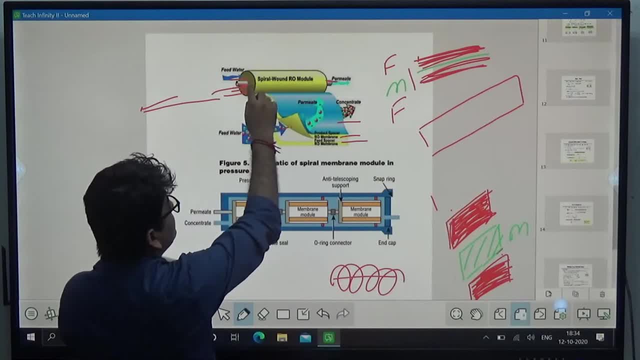 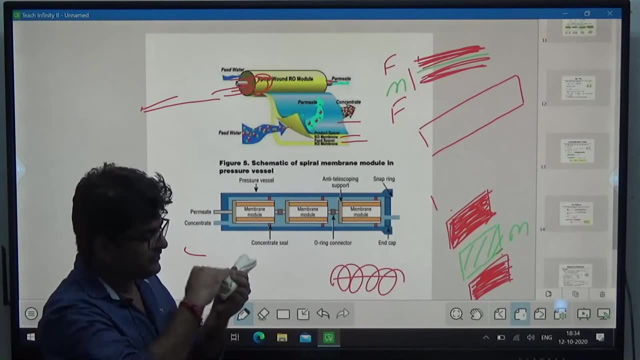 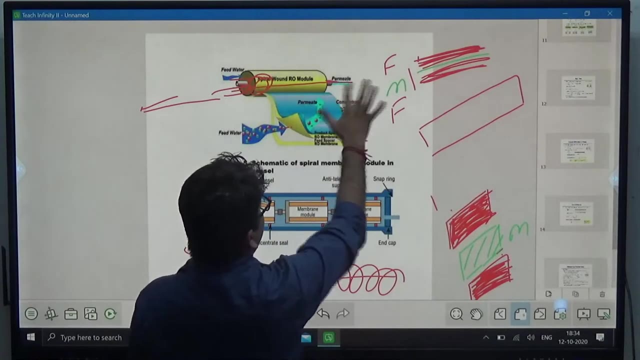 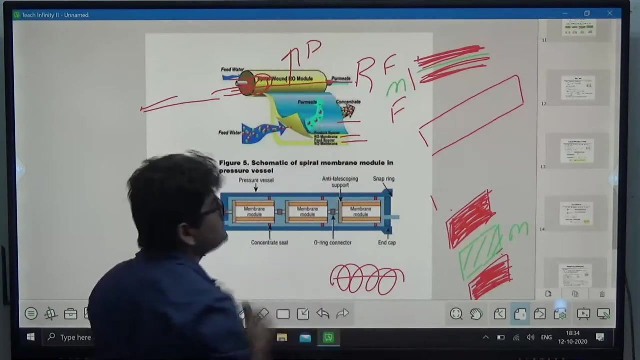 thing like this: and here, when feed will enter the selective component, the selective constituent will pass through the membrane and the retentate will remain as it is Okay. So here I will get the retentate and here I will get the permeate. okay, 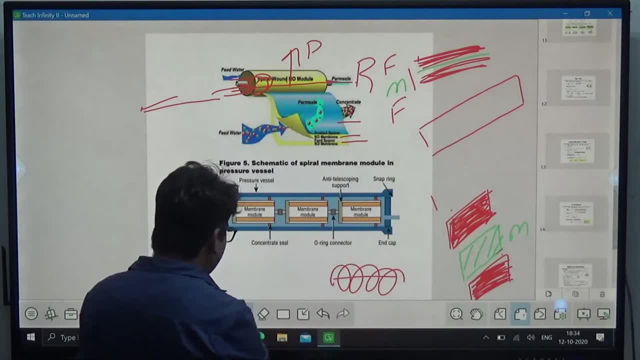 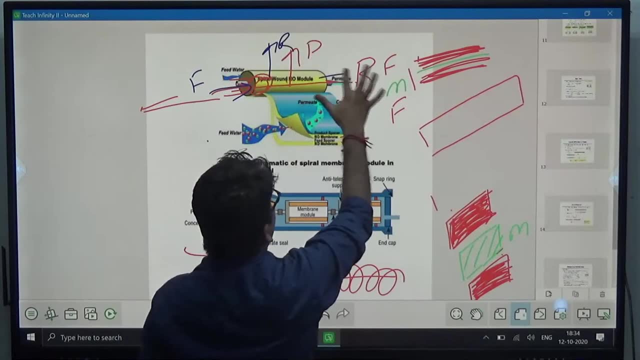 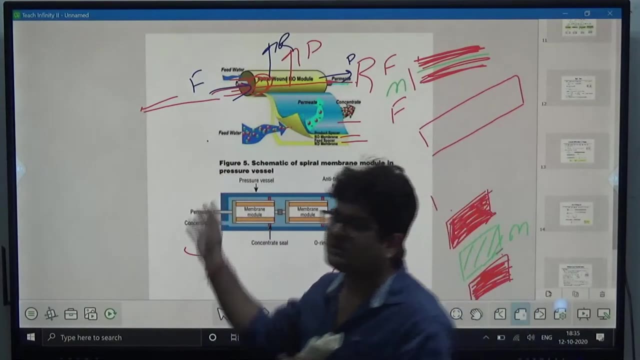 Or based on the types of flow. you can also make the design like that: I am sending feed here, I am getting retentate here and I am getting permeate here. Okay, These are the types of operation: cross flow, counter flow, current. we will discuss all. 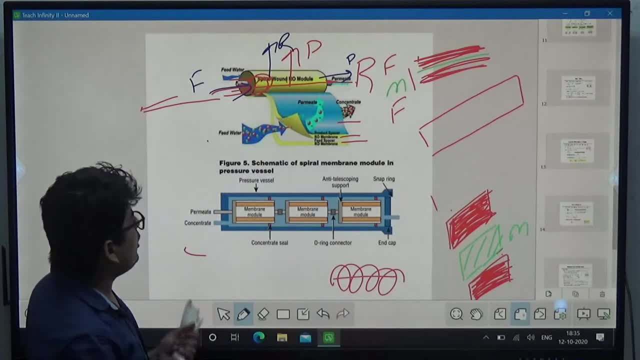 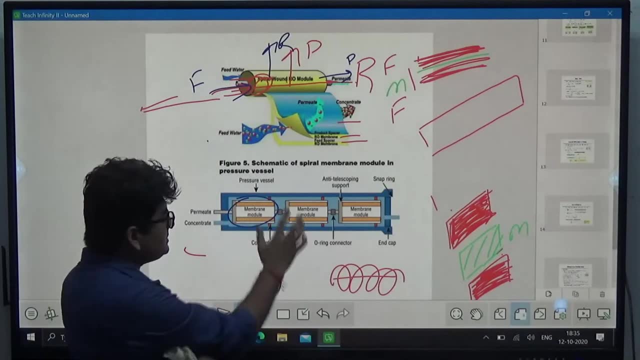 these things in the next lecture. Do not worry about that. So what is happening if you place these spiral bounds in series? this is one module, one spiral bound. this is second spiral bound. this is third spiral bound, like this: 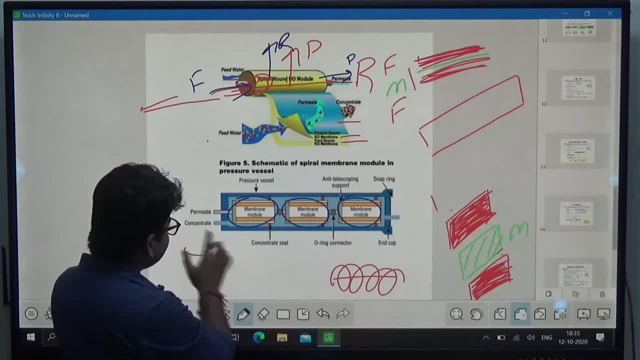 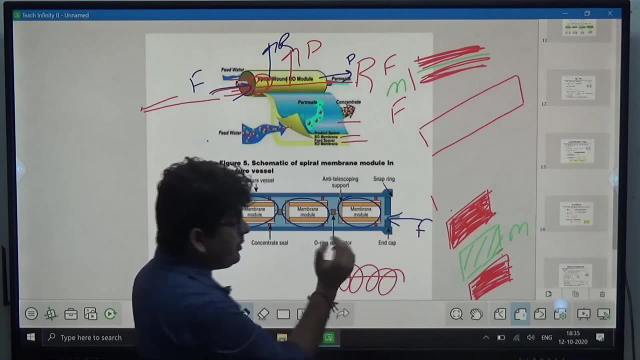 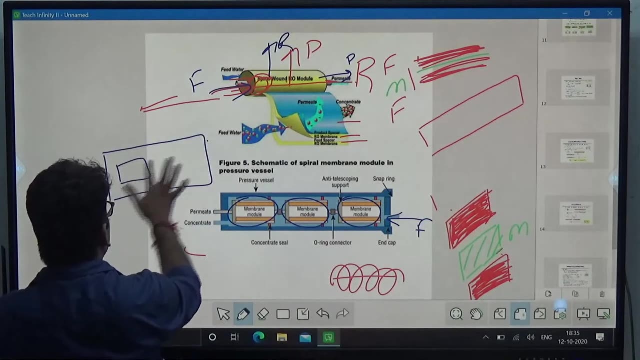 So what I am doing, I am sending the feed in this. this is the end from where I am sending the feed, just like a shell and tube heat exchanger. you can consider This is a shell and these are the modules. I am sending the feed in the shell- shell side. 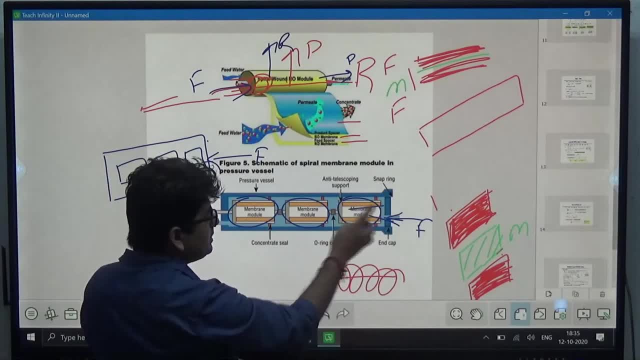 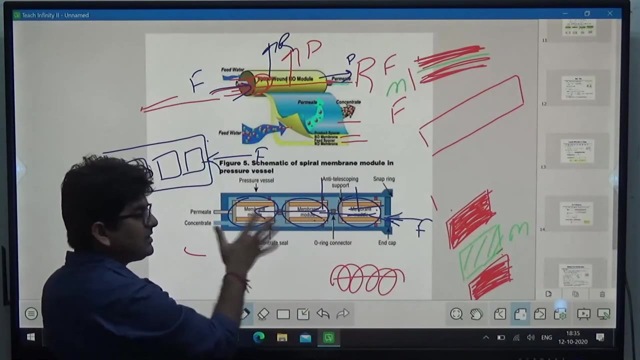 Okay, Now feed will enter in this module. separation will occur. permeate will cross or retentate will pass from one module to another module. Permeate will cross and retentate will pass from one module to another module, like this: 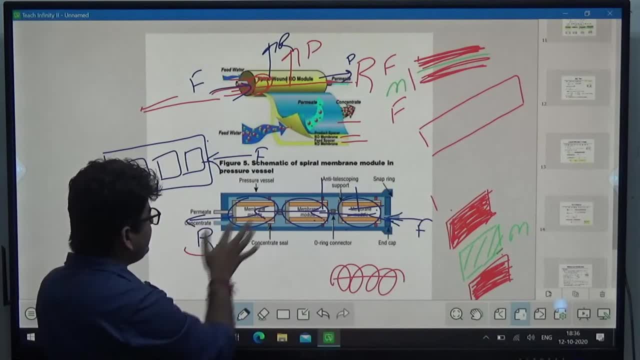 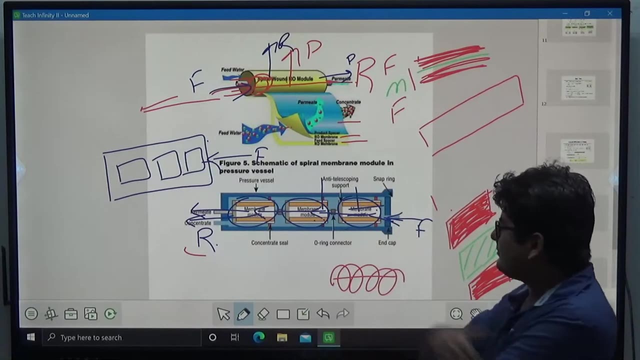 And here I will. I am supposed to get the retentate and permeate. You can say like this: whatever it is, These are the types of flow. Okay, We will discuss that thing. the counter current, co-current, Like, if I talk about this, this is the co-current flow where the retentate and permeate both. 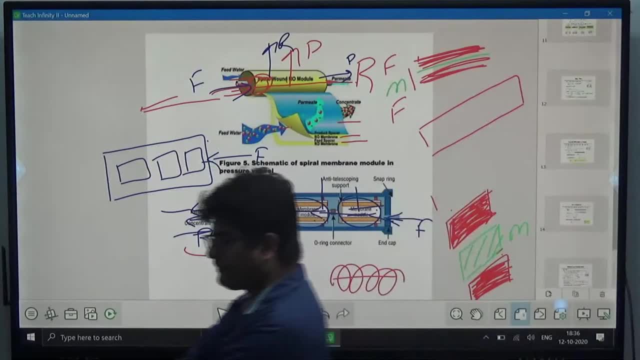 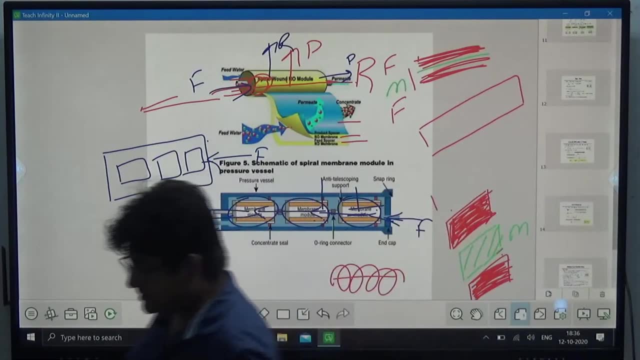 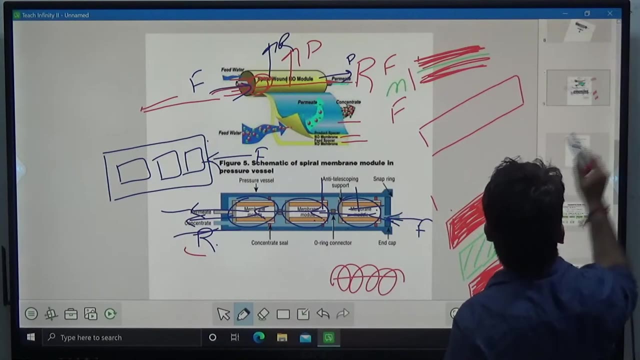 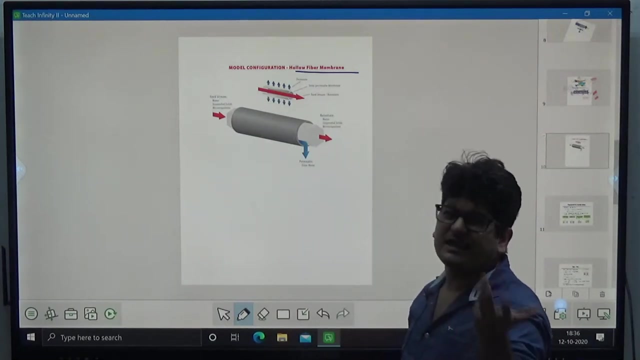 are leaving in the same direction. That is the co-current flow, or you can say parallel flow. Next is this the hollow fiber membrane. Hollow fiber membrane is, you can say, just like a shell and tube heat exchanger. Okay, We have a cylindrical shell. 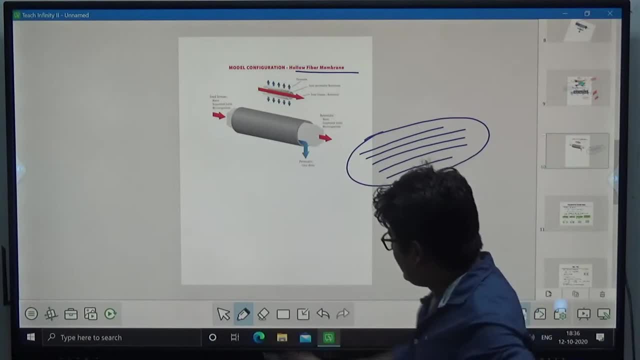 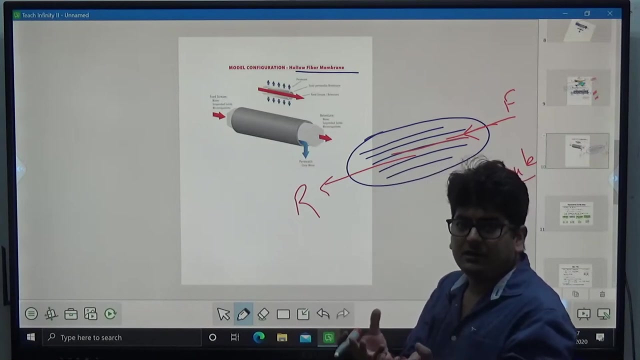 Some tubes are placed in that shell. What we do, I am sending the feed. Either you are sending the feed inside the tubes, inside the tubes, Okay. So here through the tubes, you will get the retentate. And when the feed enters inside the tube, obviously membranes are there attached to. 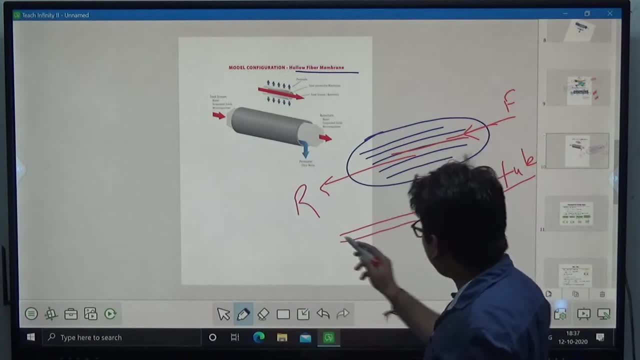 the inner walls of the tube. This is the tube. Membranes are attached to the inner walls of the tube. Feed is crossing, Permeate will pass And here I will get the retentate. So permeate I am getting. 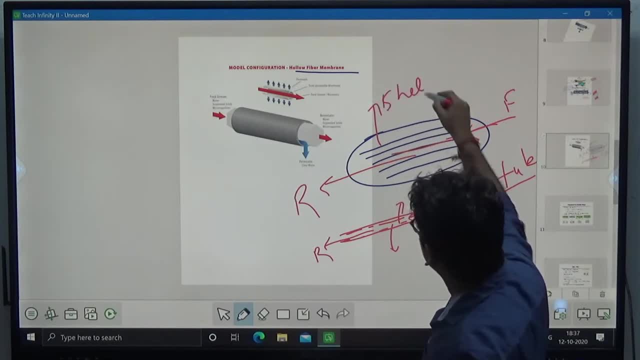 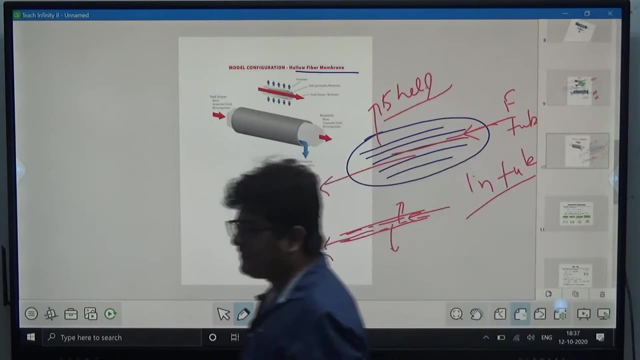 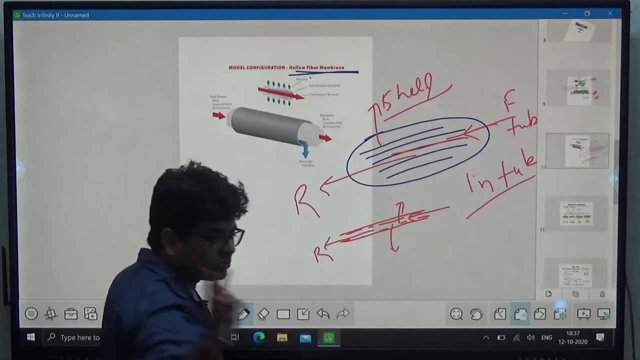 Through the shell side. If you send the feed in the tube you will get the permeate in the shell. Okay, That is one working Second module. second configuration is: see guys about the hollow fiber membrane. there are two types of configuration. 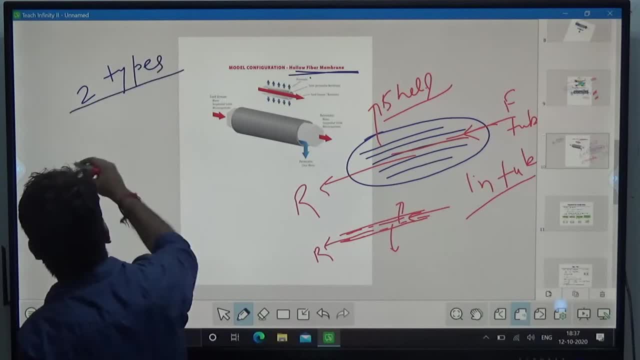 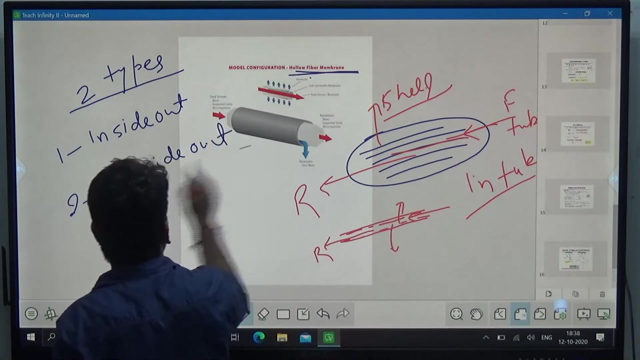 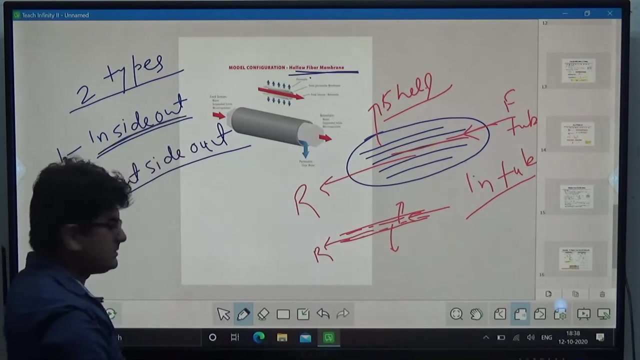 Two types. First is inside out. Second is outside out. Inside out means if this is a cylindrical and shell assembly, like this Cylindrical shell and these are the tubes. Okay, So here, what will I do? I will send my feed in inside out assembly. 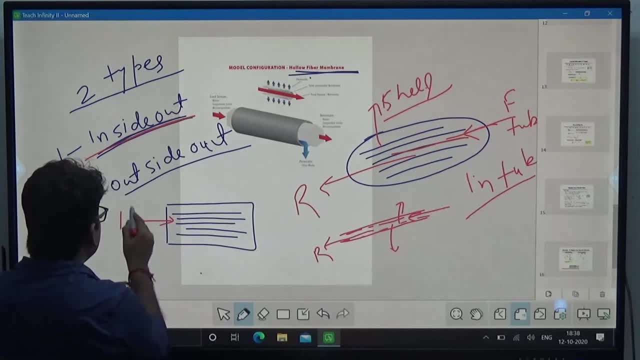 I will send my feed inside out assembly. I will send the feed in the tubes In tubes, So feed will enter inside the tube, Feed will flow inside the tube, Permeate will pass And here I will get the retentate through the outlet of tube. 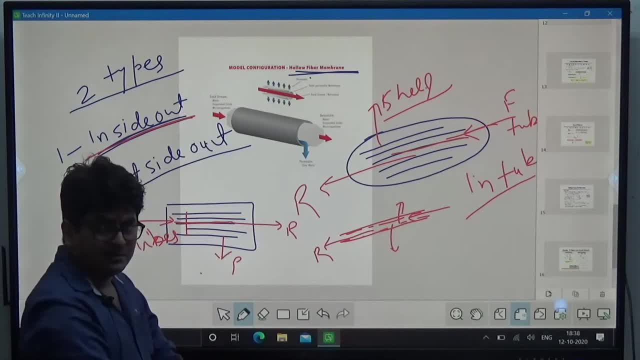 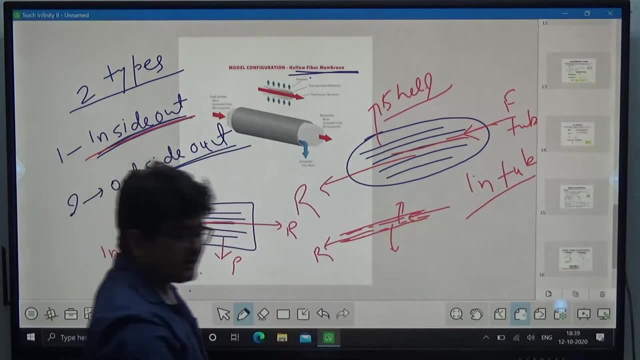 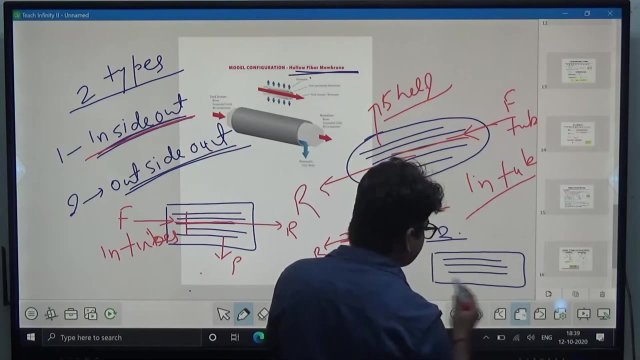 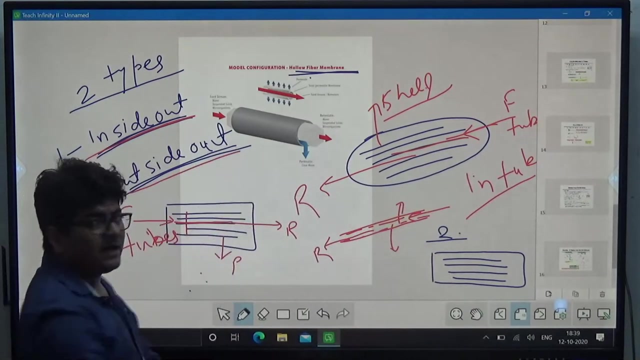 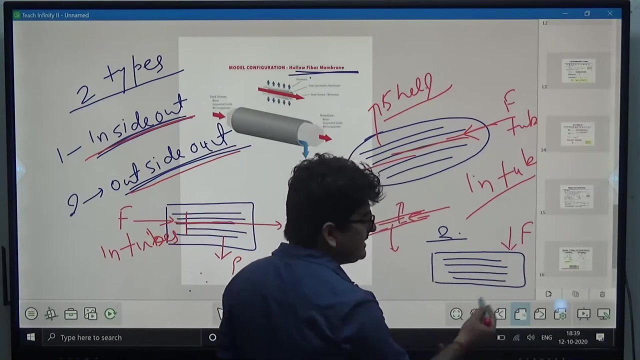 and I will get the permeate through the outlet of shell. that is the inside out arrangement. Second arrangement is outside out, where what I do suppose this is the cylindrical shell, these are the tubes. so what will happen in case of outside out arrangement? outside out configuration? I will send the feed in the shell. I will send the feed in the shell, okay. 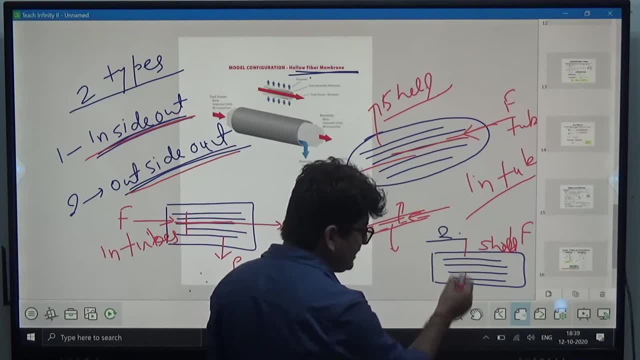 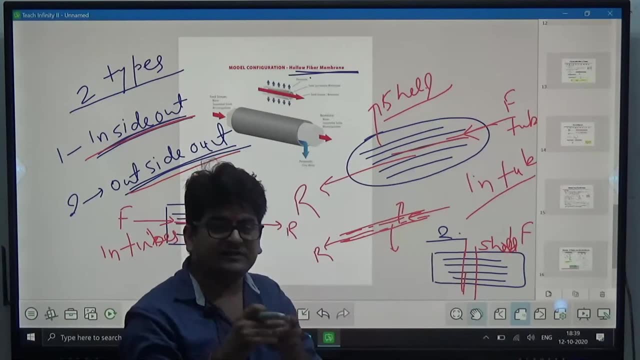 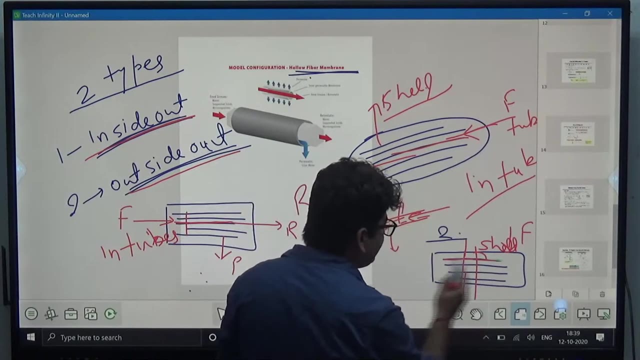 so feed will pass through the shells, feed will flow in the shell. so what will happen? permeate will pass the constituent which is getting separated. it will move inside the tube. the permeate will move inside the tube and I will, and I will get the permeate through. 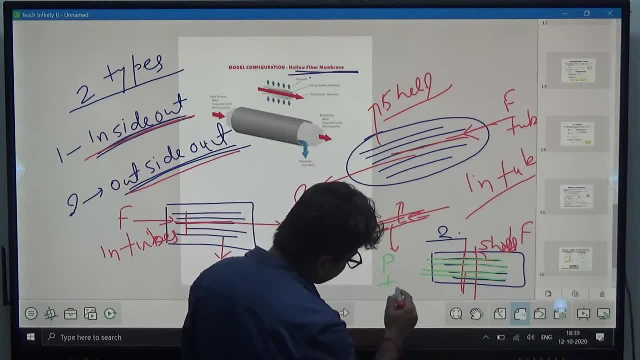 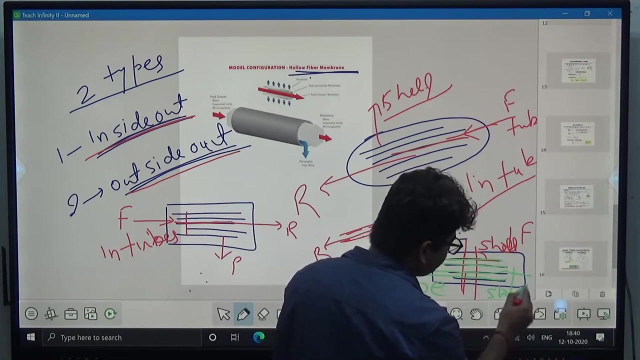 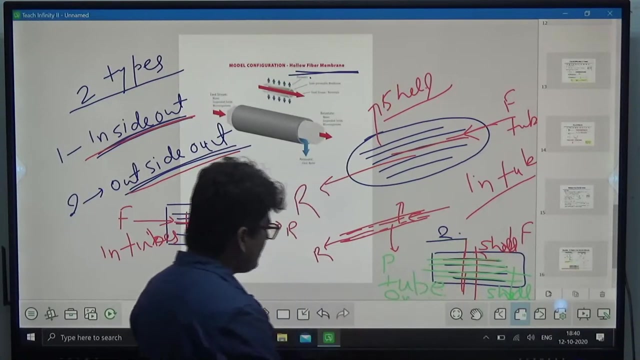 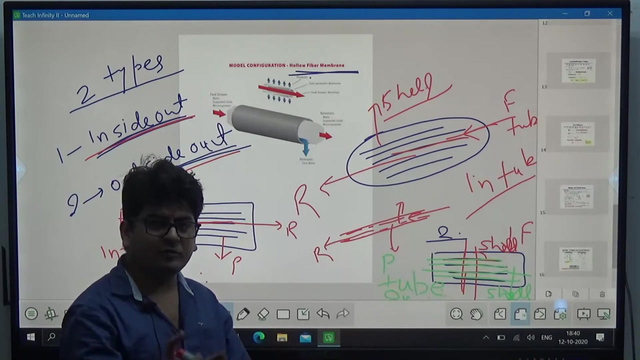 the tube outlet. I will get the permeate through the tube outlet and the feed will leave from the shell side. Okay, like in shell and tide heat exchanger, either you can send the hot fluid in the shell or you can send the hot fluid in the pipe tubes. 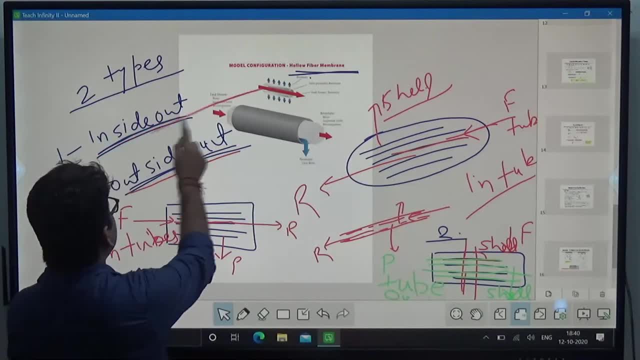 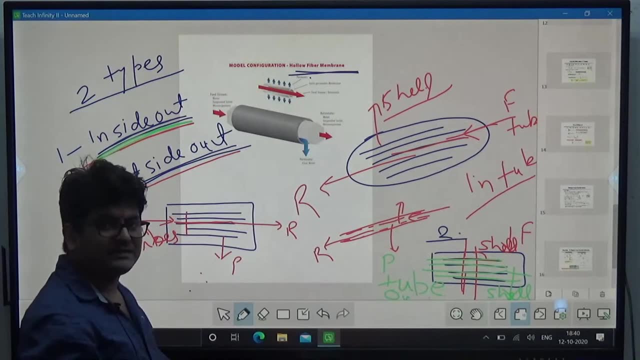 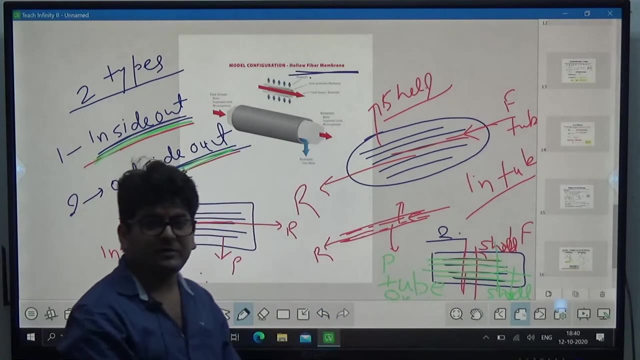 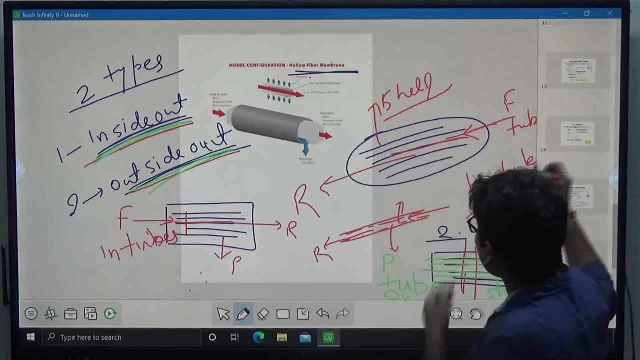 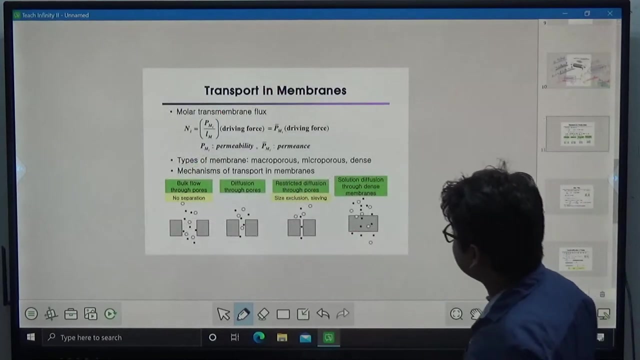 So similarly here. inside out means you are sending the feed, you are sending the feed inside the tube and you will get the permeate from shell side. Outside out means you are sending the feed through shell side and permeate you will get get through the tube side. okay, this is the hollow fiber arrangement, guys. 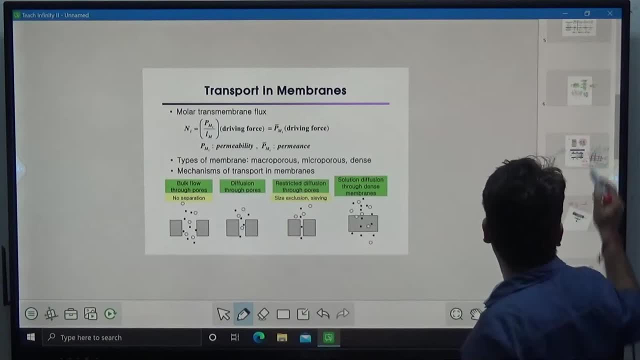 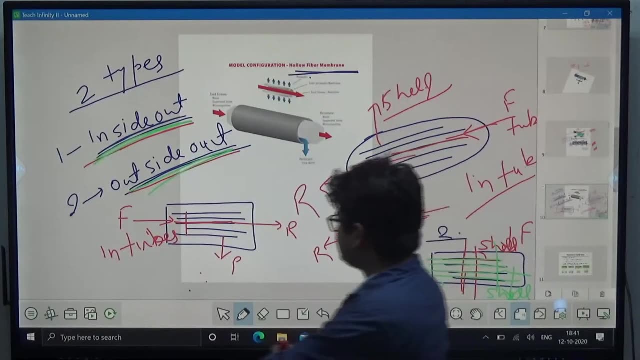 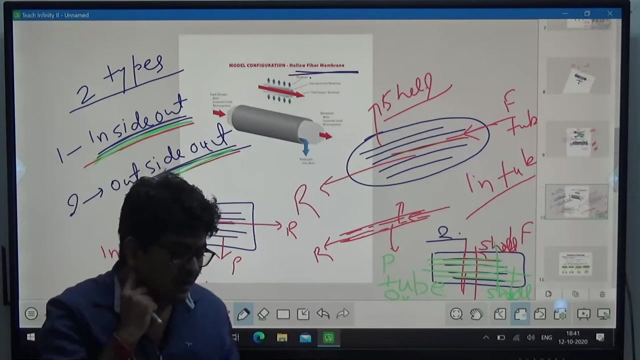 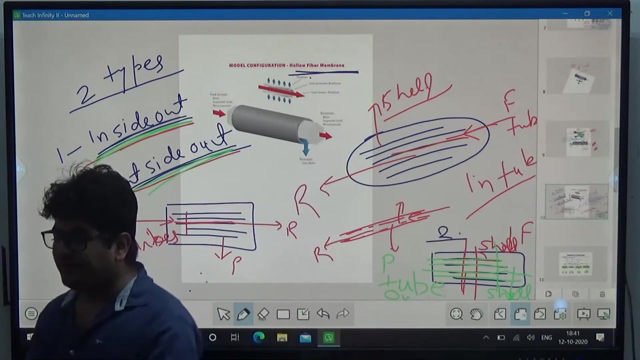 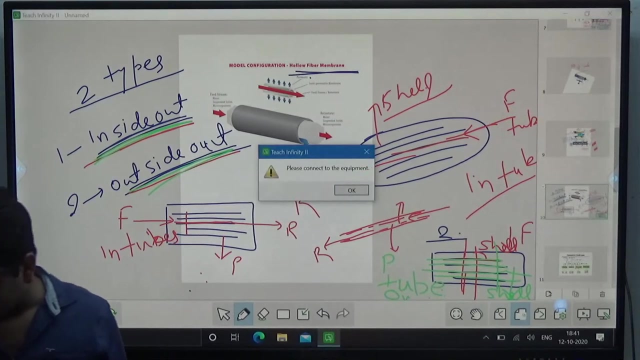 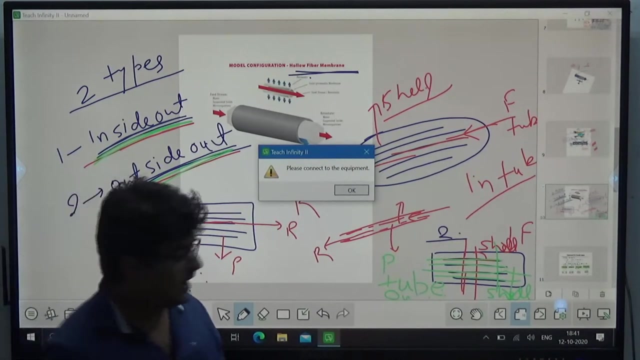 transportation. that is a different thing, so we should not talk about that here. so i hope this is clear to all of you. about the membrane modules, how they are working. okay, now the next part is the applications: the advantages, disadvantages of all these membrane modules, and one more thing about them is the selection. 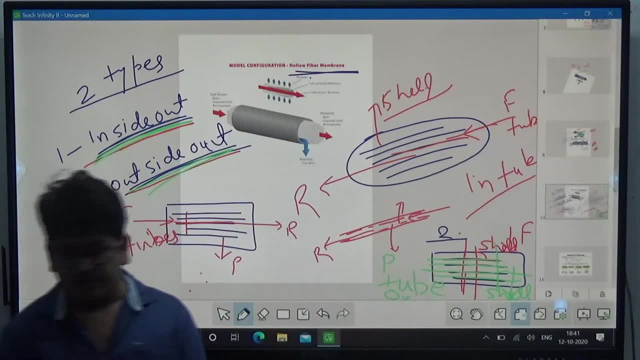 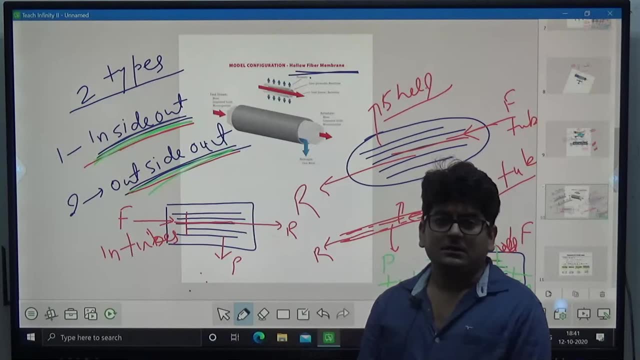 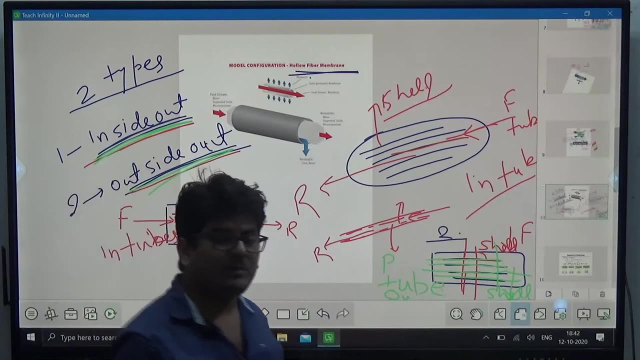 the selection of the membrane modules. okay, so it's very easy to understand about selection of anything like at your home as well, if you are planning to purchase any refrigerator, or you are planning to purchase any computer, for example, so, or any mobile. so you go to any shop and you say that to the shopkeeper: i want to buy a. 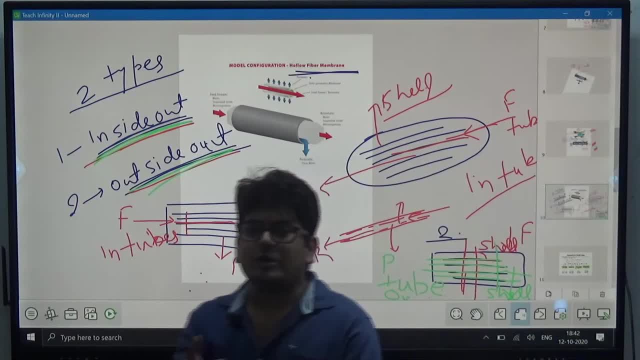 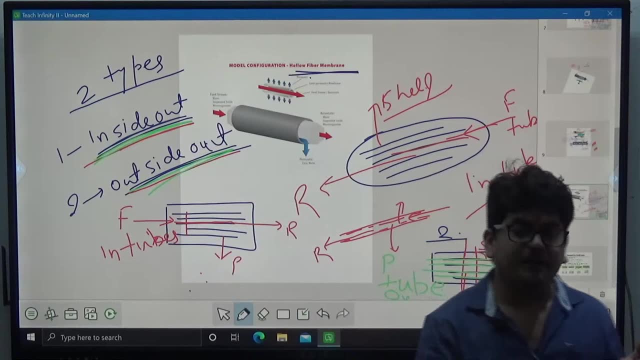 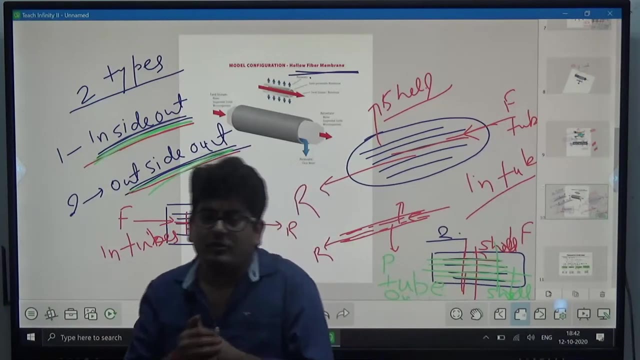 mobile. okay. so he asks you: what are your requirements? okay, so you say that first requirement is obviously the budget. second requirement is the use, like if you are purchasing any mobile, for example, your grand grandparents- okay, those people are so old that normally they don't want to use any whatsapp telegram. 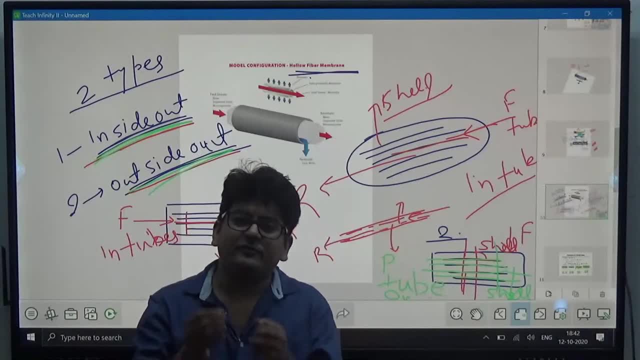 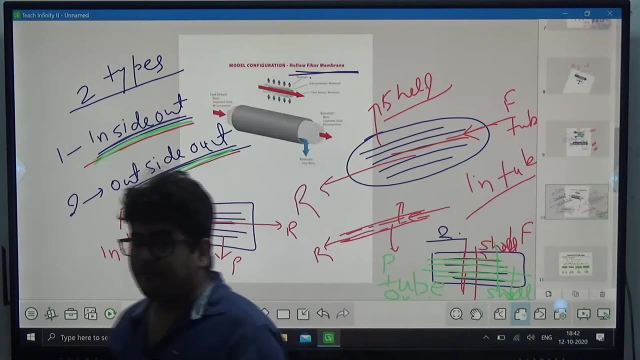 or anything, okay. so they just want a mobile phone for calling purposes. so what will you say? i want this mobile for calling purpose only, So you will go for the Nokia classic phone or the Samsung small phones, like that Java application based mobile, Okay. But if you are purchasing, 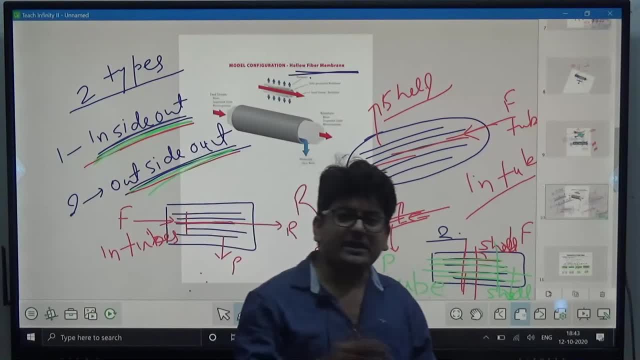 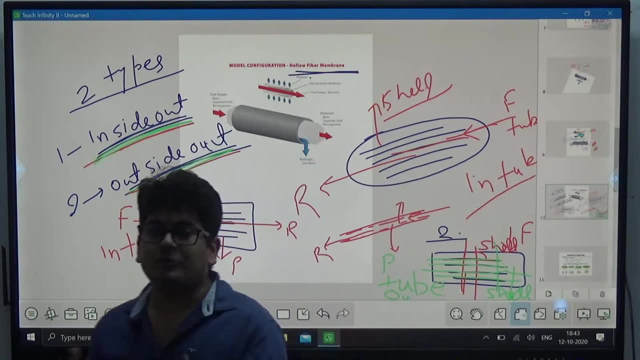 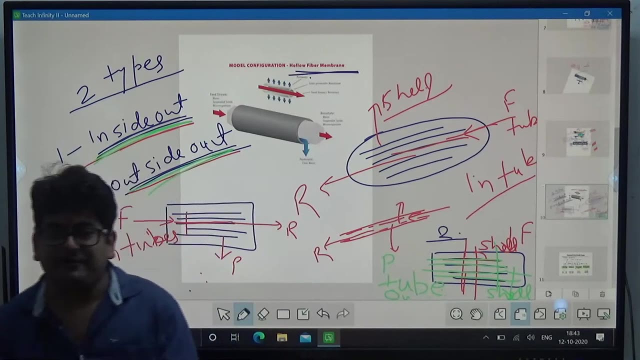 a mobile for yourself, then what will you say? I want a mobile like. if your hobby is computer gaming, then you will say that I want to play computer games or, sorry, mobile games. So give me a mobile which will have the highest configuration, like a very large. 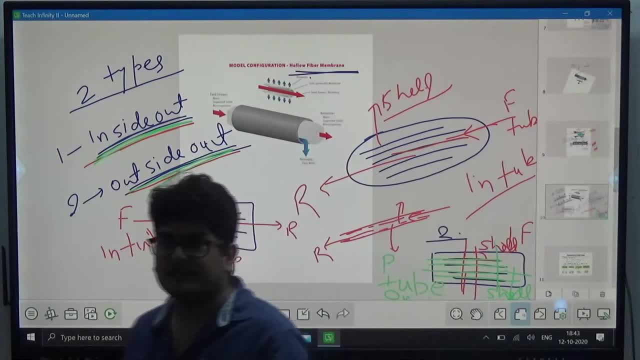 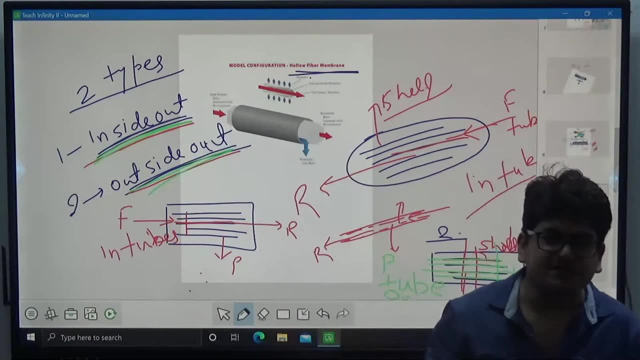 size, RAM, a very storage capacity should be high, all these things. Touch should be very comfortable, smooth, Gyroscope feature should be there. All these things are there. Motion sensor, You will say like that. So similarly when I talk about the membrane modules, so 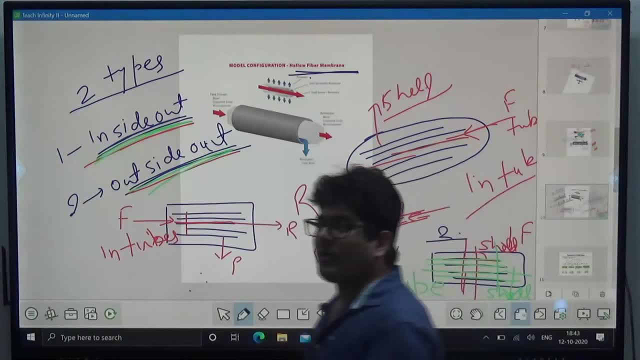 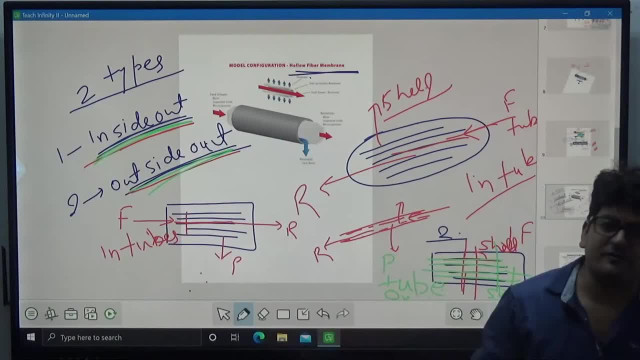 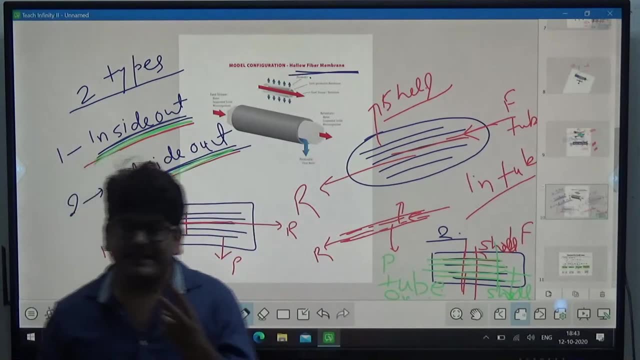 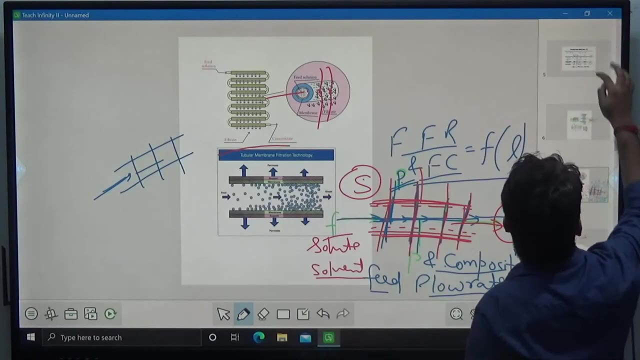 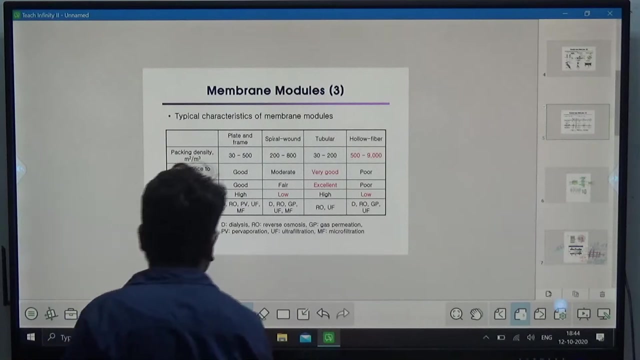 The second requirement is the cost. Okay, The initial cost of the membrane module. Initial cost means the fixed cost, the purchasing cost of the membrane module. Second is the packing. As I told you this, the requirements are like this. You can see Cost ho gaya cost. 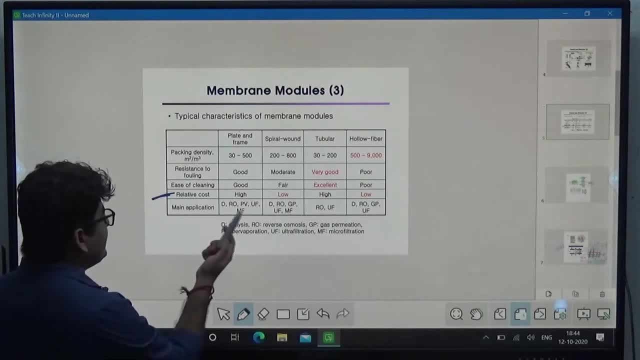 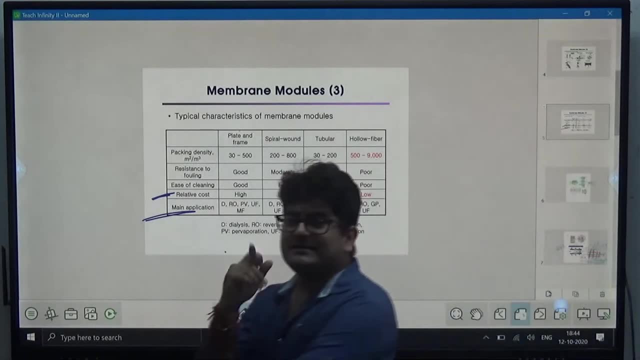 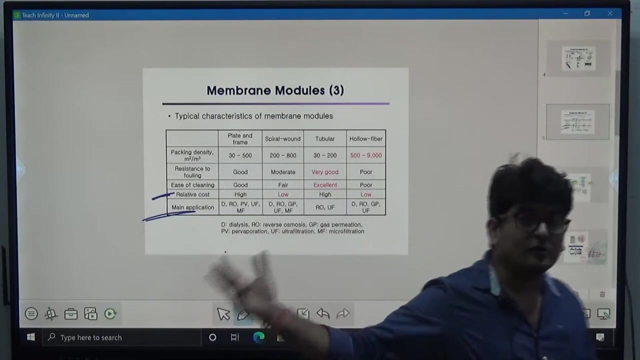 ho gaya. You can see the relative cost. Second is the application: Why you are you what you want to do? the membrane module, For example. you want to purify any water, like at our like, as our, in our households, we use the membrane separation technique, membrane- 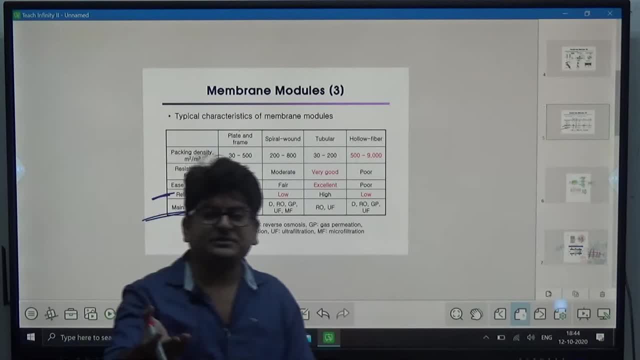 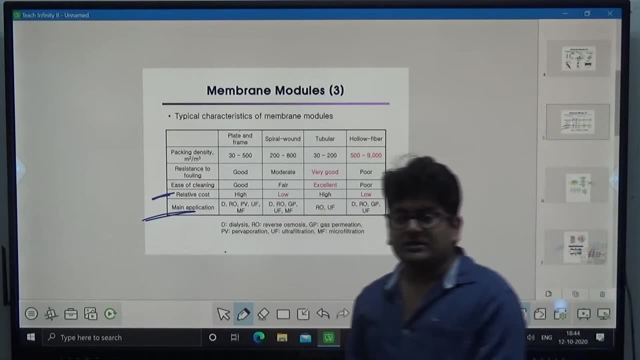 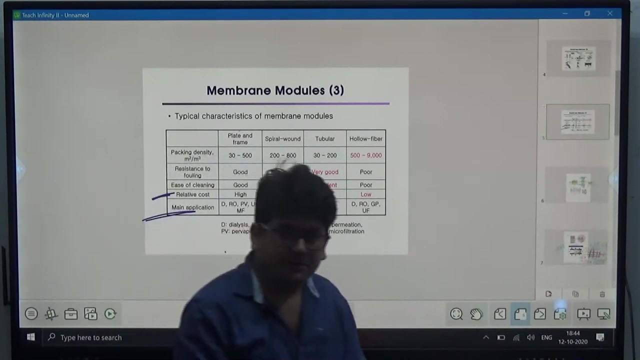 separation processes for the water purification purpose, which normally we use- RO systems, reverse osmosis systems, Okay. Or if I talk about the membrane module, we use the membrane separation process in our hospitals. So they use the membrane separation processes in dialysis as well, where they want to purify the blood. Okay. One more thing is one more. 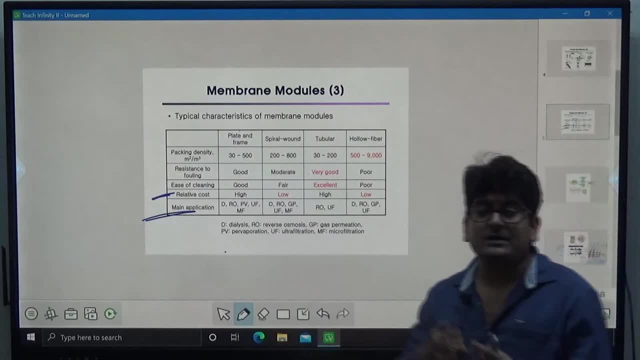 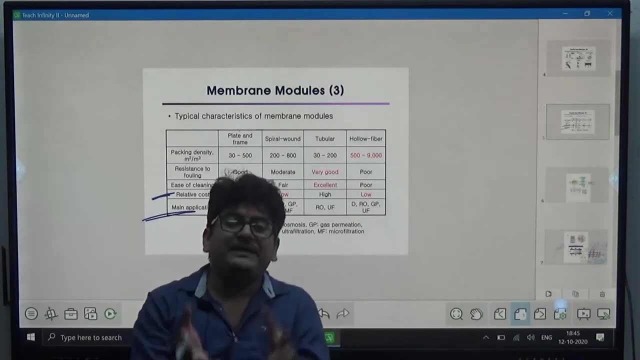 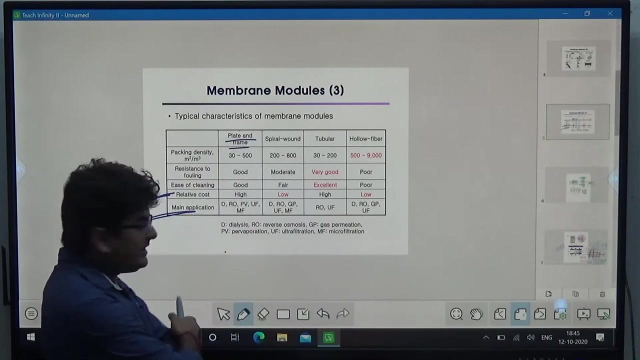 application where they want to separate the plasma, hemoglobin, all these kinds of things from the blood. So that is one other dialysis operation. So depending on those requirements we use the membrane module like plate and frame membrane module we can use for the. 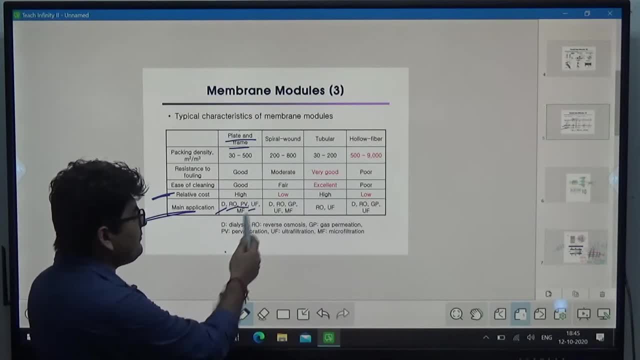 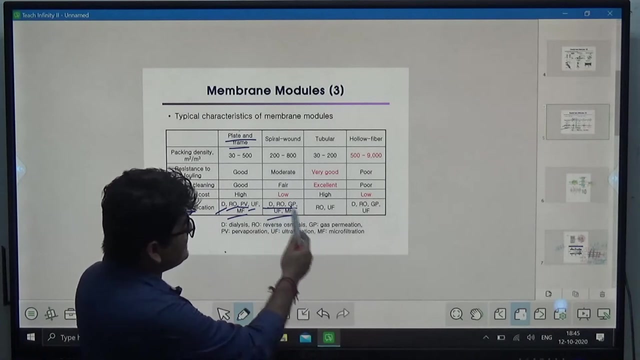 dialysis, reverse osmosis, pervaporation, ultrafiltration, microfiltration. Okay, Spiral wound membrane we cannot use for the pervaporation purpose, So we can use that only for dialysis, RO, gas permeation, ultrafiltration, microfiltration. Tubular membranes: we can use only for RO or 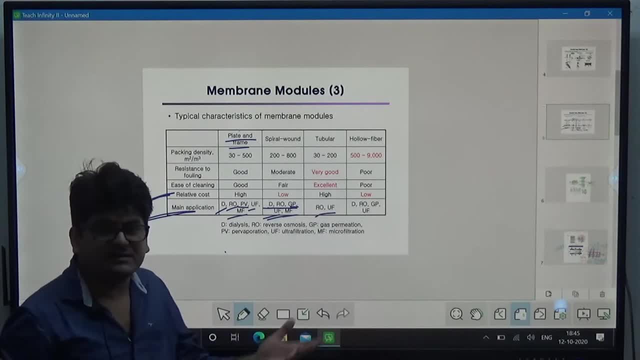 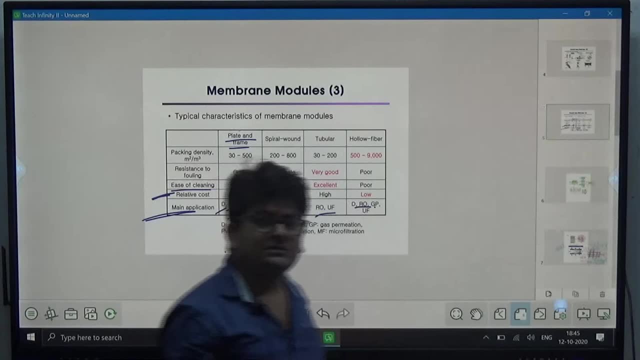 ultrafiltration, even not for the microfiltration and other stuff. Okay, And like, this Other thing is cleaning, After all. next, what I want, I want to clean the filter, the membrane. Okay, You know that, after a long run of application, long run, 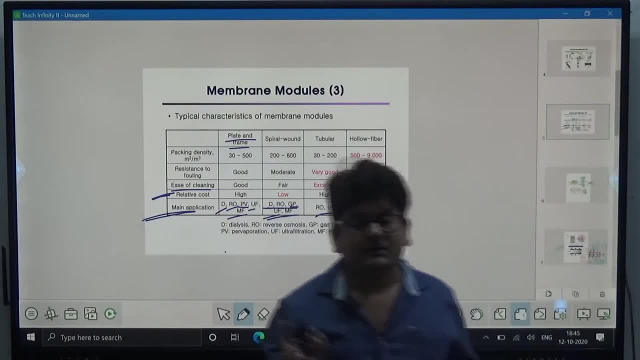 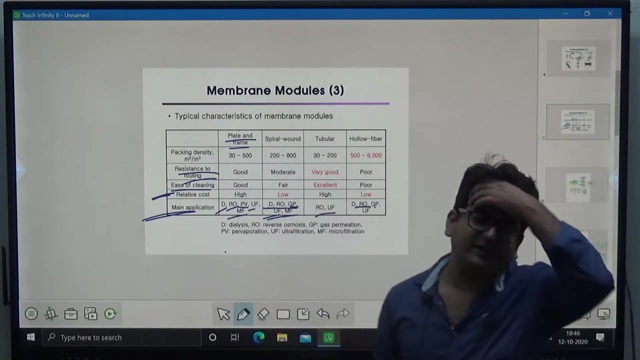 of process, the fouling may occur. Fouling means some solid particles may get deposited on the surface of the membrane. So obviously I want to clean that. the maintenance cost- So it should be low, depending on that. What is the quality? If I talk about the hospital in the medical industry, there I want to purify. 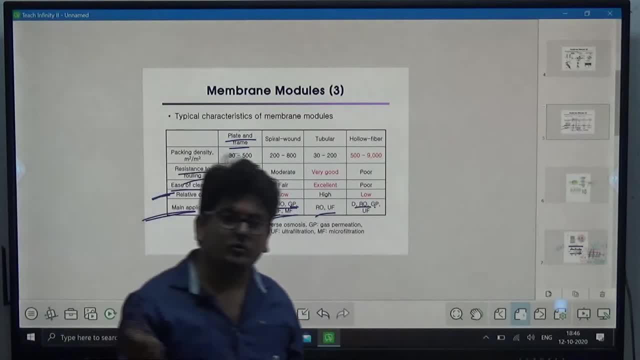 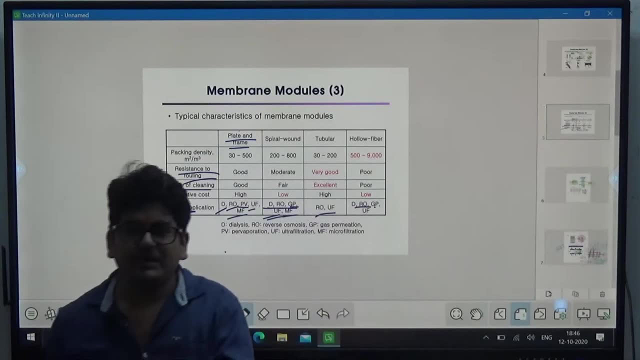 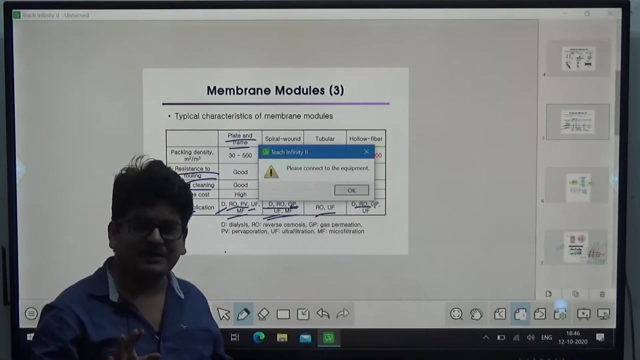 the blood. I want to separate the plasma, hemoglobin, other stuff, WBC, RBC, what are the things are there? I don't know. You know better than me, So you can understand. Okay, I just know one thing: that blood, human blood, can be divided into four categories. We can: 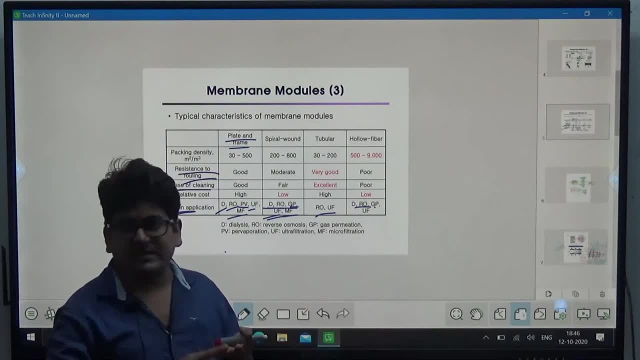 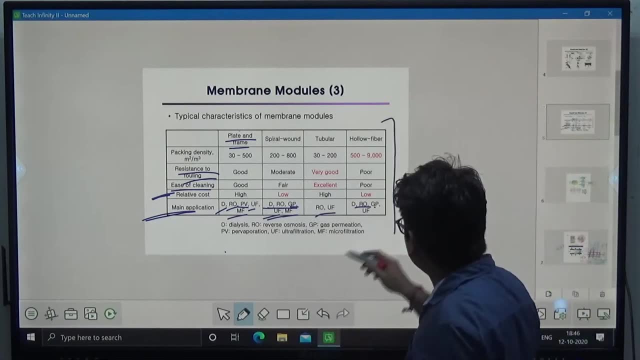 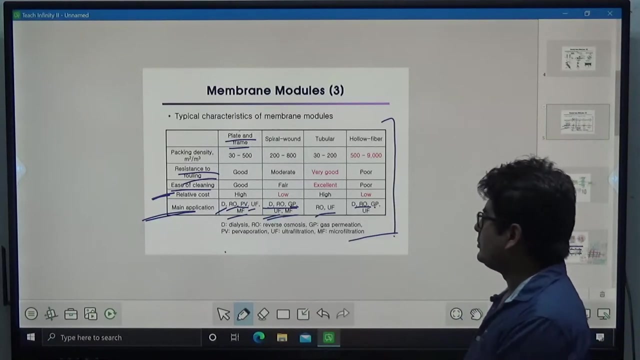 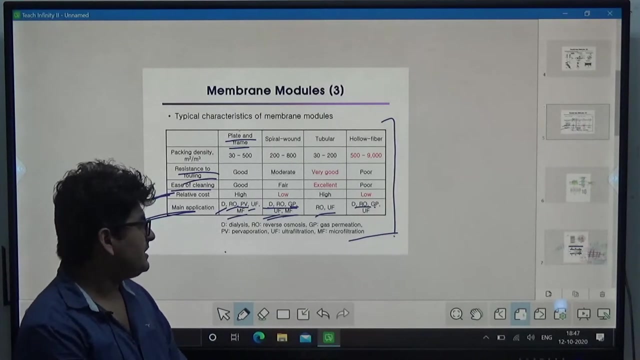 get hemoglobin, We can get plasma And two more things are there that I don't know. Okay, I forget all that stuff. Fortunately, I didn't require to go into the hospital, So I forget all that stuff. So, depending on that, obviously you will not use that type of separation membrane. 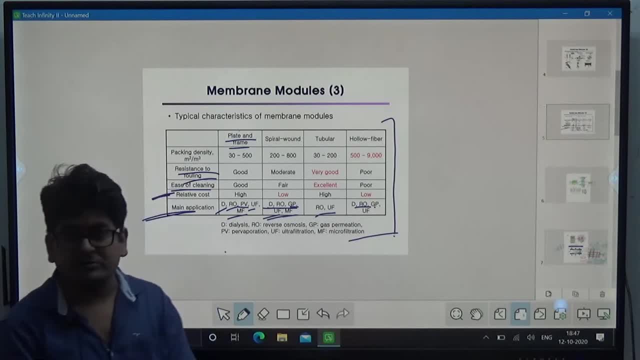 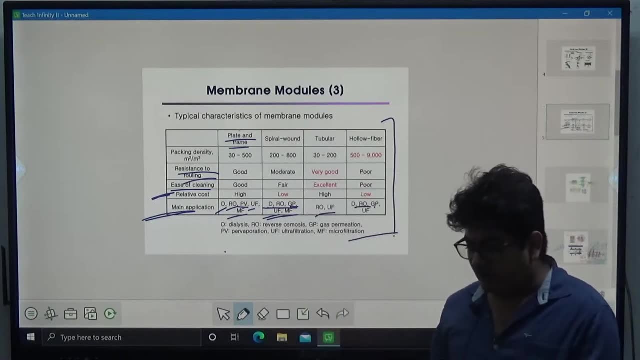 separation equipment at your home, Because at your home you don't want to separate the blood, You just want to separate the water. So let's talk about the industry. So, based on the water purification as well, there are two types of equipment, Like if I talk about the households. 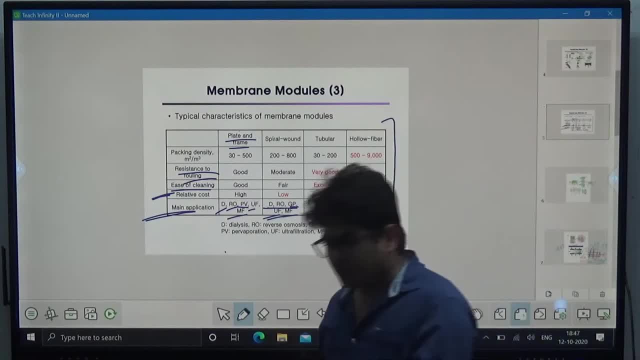 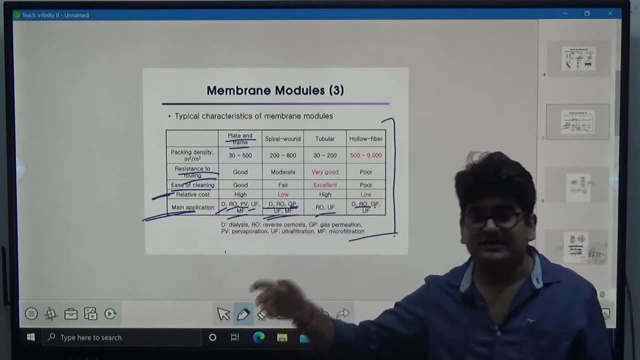 in our households we are getting the water from the ground, So that groundwater we want to separate, we want to purify. But if I talk about the industries in industry, they are getting the water from the ground as well, as some sea water is also getting the water from the ground. 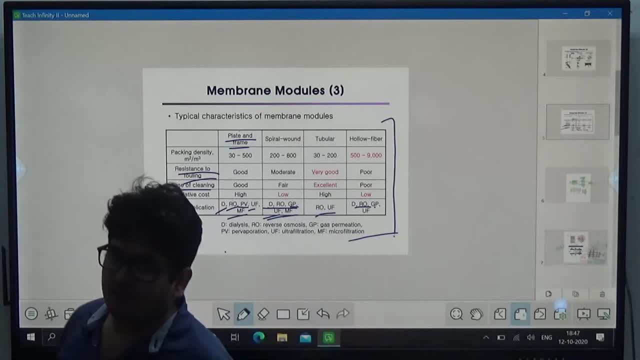 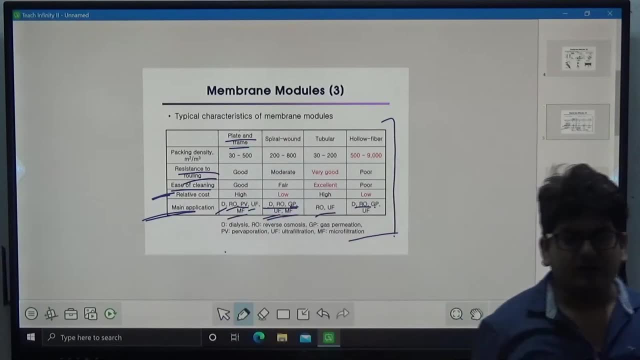 Okay, From that they are purifying the water desalination processes. you can say or otherwise the membrane distillation process. These are some different things. So I hope, guys, it is clear to all of you What are the requirements, What are the selection criteria to separate. 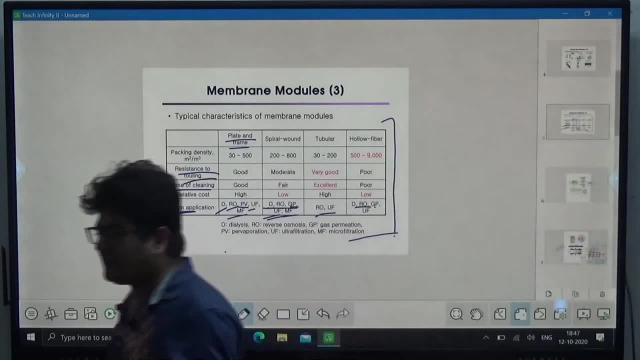 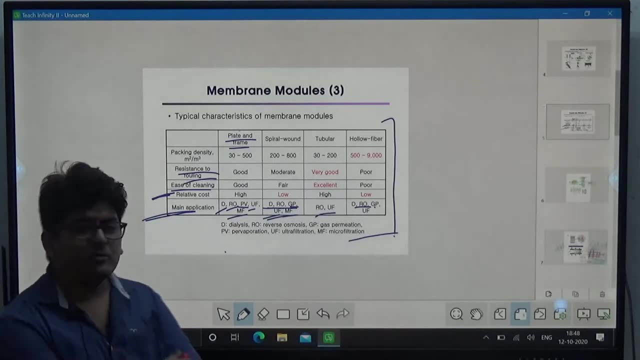 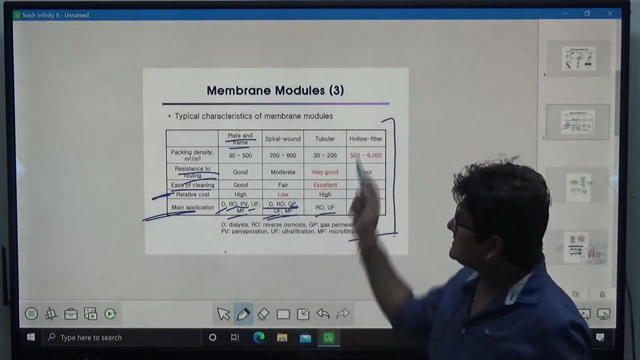 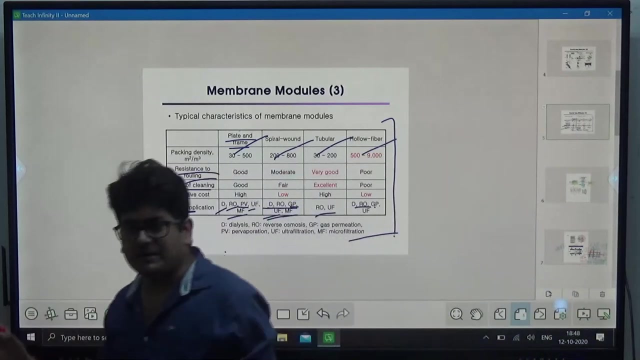 a membrane module. It is very simple to remember. Okay, That's not a big deal. So this is all about the membrane module guys And the advantages, disadvantages and applications of all these modules: platen, frame, spiral bound, tubular, hollow fiber. you can see in the PPT or in the telegram group. I will share that. 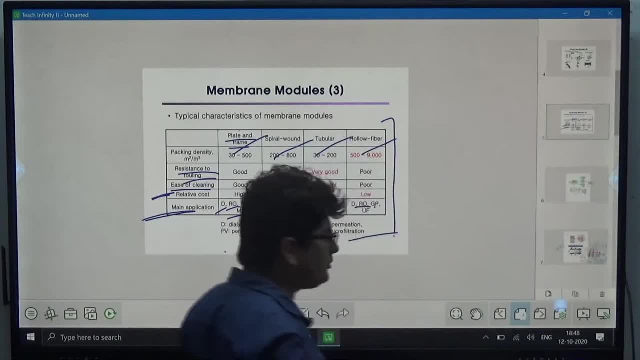 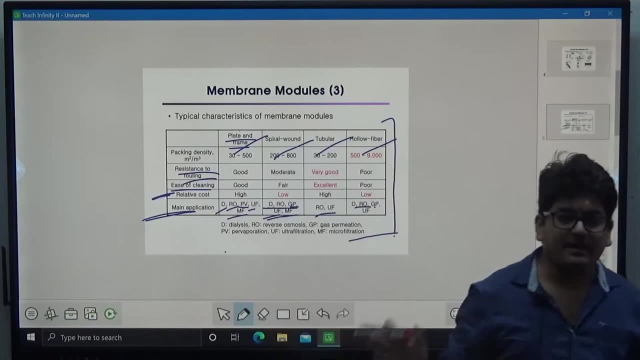 today evening, By today evening, you can watch, you can memorize all those theoretical parts. Next, the important part in the membrane separation, the only important part in the membrane separation which is not theoretical only, that is the numerical based, mathematical best, that is. 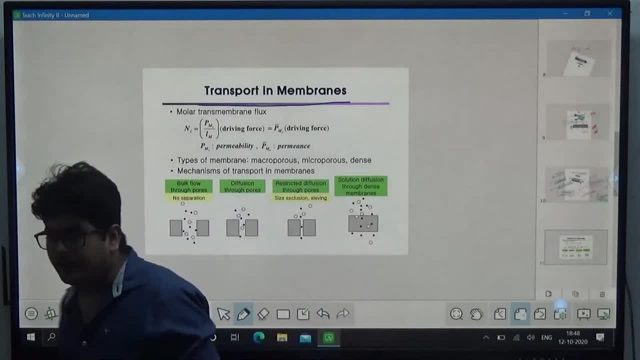 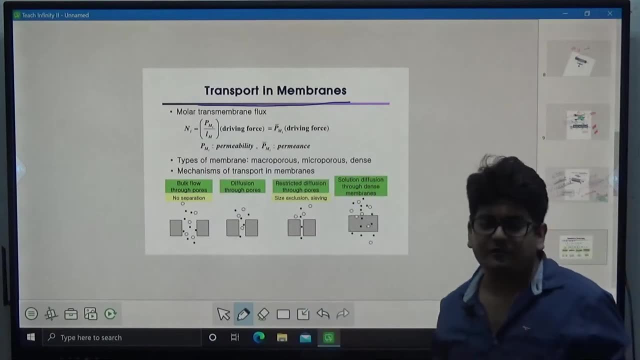 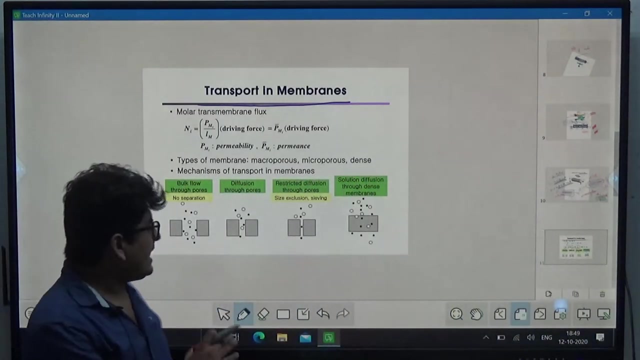 that transport theories in membrane. Okay, So I hope you know the fixed first law of diffusion. Okay, We will discuss all the transport theories Here. I am just giving you one recap, or you can say pre-cap. Okay, we will discuss about the transport theories on Wednesday or Thursday. 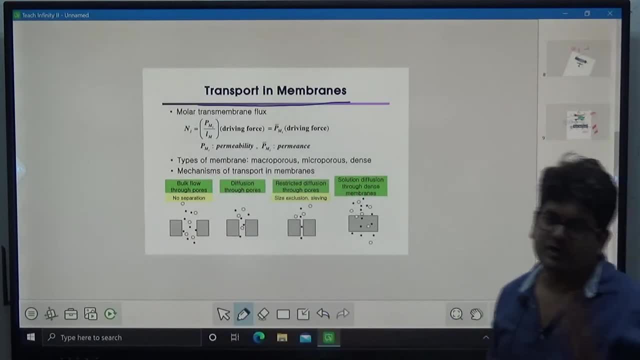 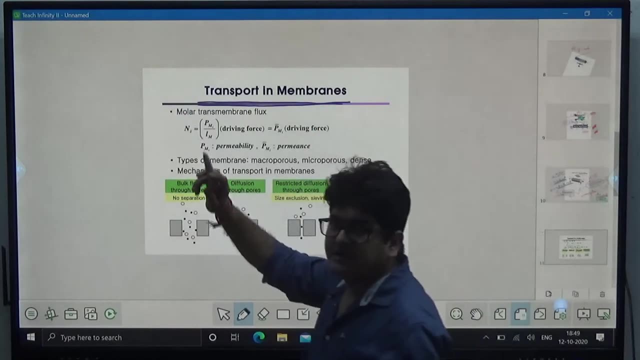 Tuesday I will share the schedule till tomorrow. you can watch that on our page or in the telegram group as well. So transport theories we will discuss in detail, where you know that this Ni is the flux driving force and normally we define the flux as driving force over resistance. 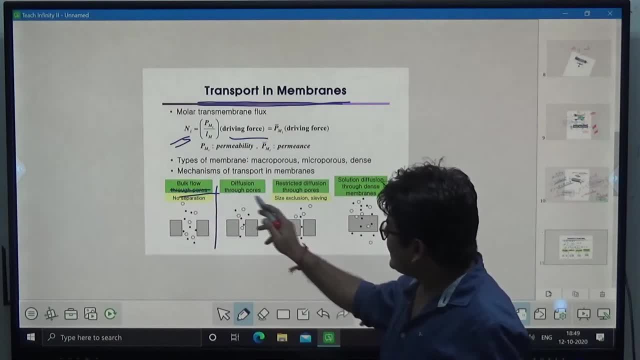 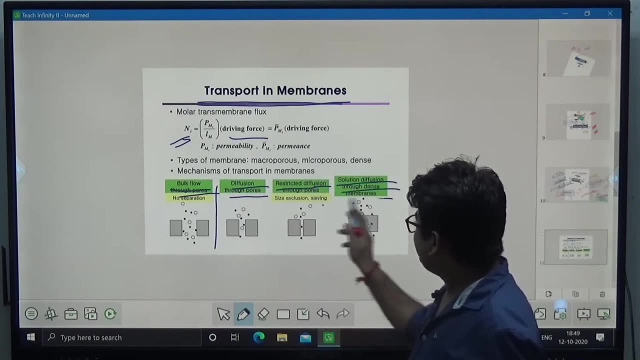 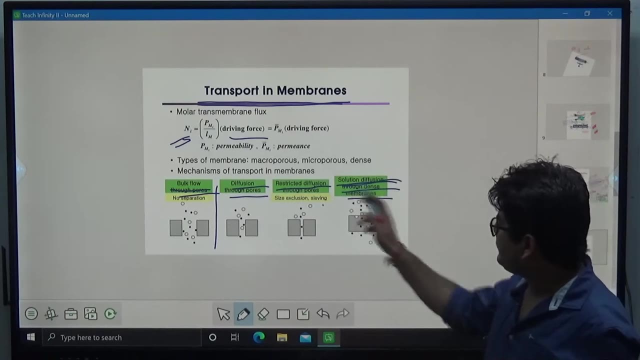 These are the theories: bulk flow through pores, second is diffusion through pores, third is resist restricted diffusion and the fourth one is solution diffusion method. So here mainly we will talk about the two theories. one is solution diffusion theory, second is bulk flow theory, Because I have seen the literature. they have also shared the detailed, they have done the 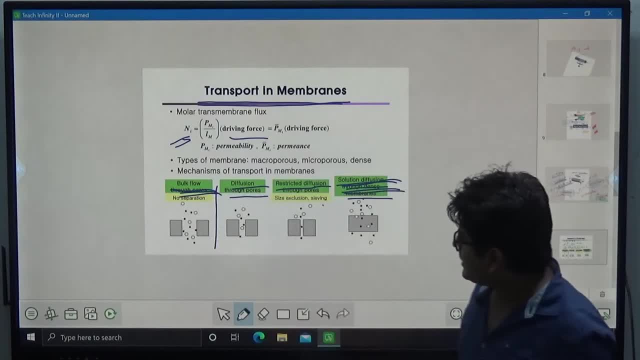 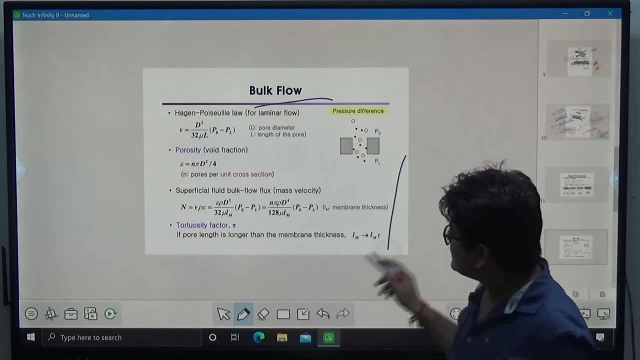 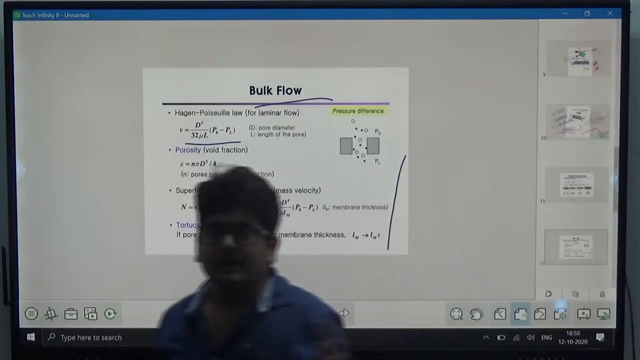 detailed discussion about these two theories only After that. this is the bulk flow theory, Guys, which we will discuss. I hope you know the Hagen-Kosley equation, as in membrane modules you have seen that in tubular flow, in hollow fiber flow membrane modules fluid, the feed is flowing through. 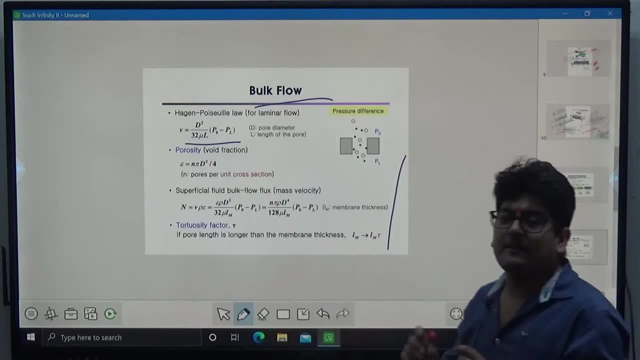 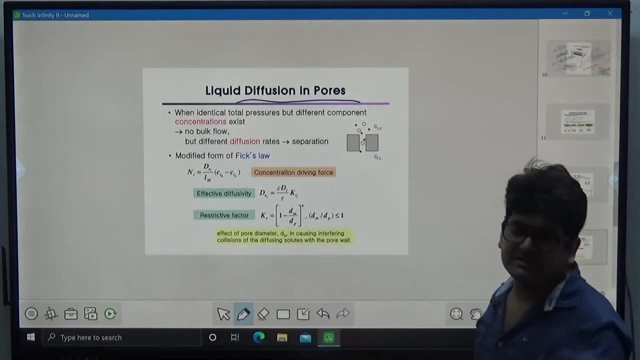 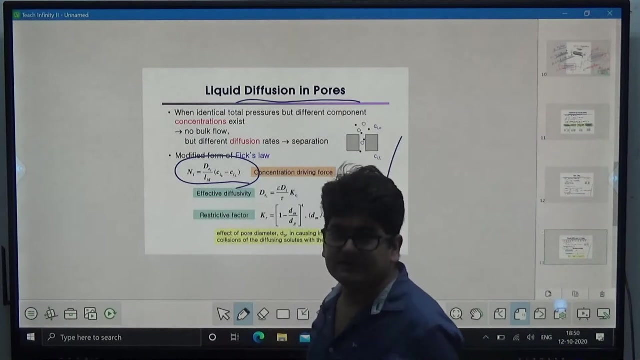 the pipe flow through the tube, through the capillaries. This is the solution: diffusion theory, or you can say liquid diffusion theory. so we will discuss about all these stuff in detail. Thank you, It is just like the mass transfer theory. if you know, in mass transfer we discuss that. 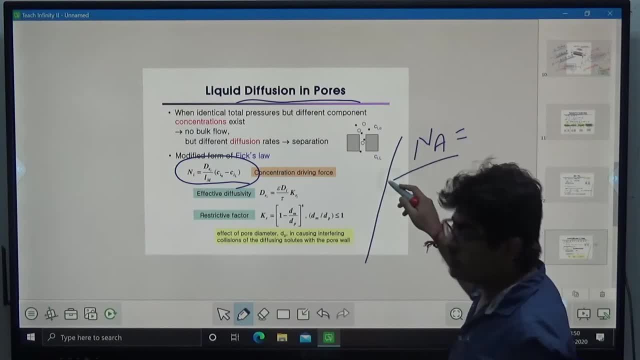 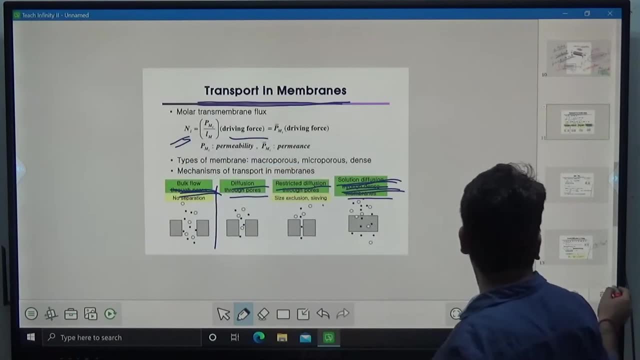 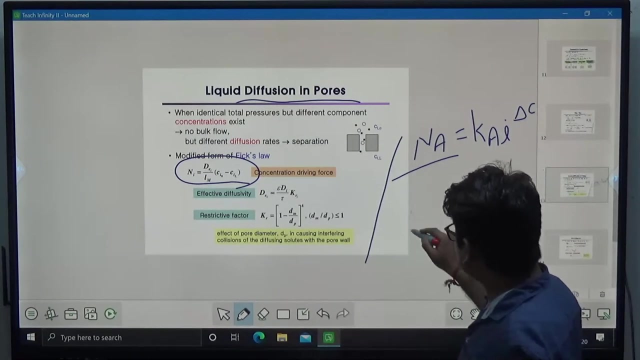 the flux. the molar flux due to bulk motion is equal to mass transfer coefficient multiplied by concentration difference, delta C. and according to first law of diffusion, the molar flux, molecular flux, is like this: This is the diffusion coefficient. here we do not talk about the diffusion coefficient. 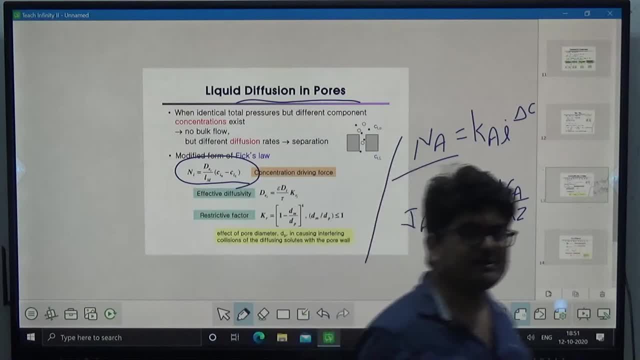 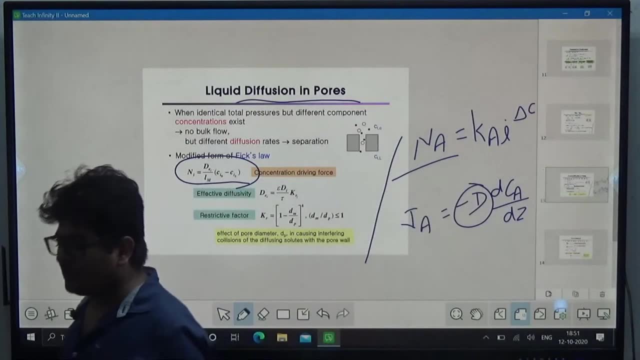 here we talk about the permeance. Permeance is basically, you can say, the coefficient of permeability. what is that? all that part we will discuss in detail in next lecture, where we will talk about the transportation from theories in membrane, and that will be the last topic, guys, in the membrane separation. 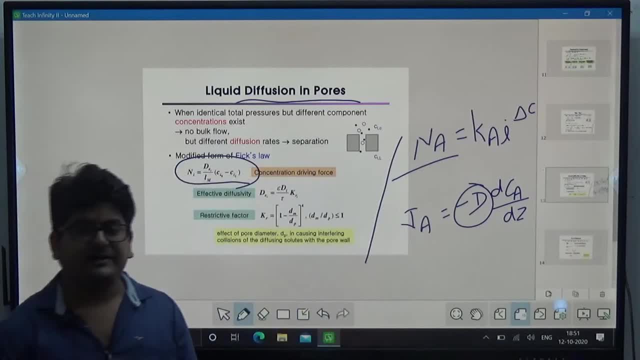 part, last lecture in the membrane separation part, and we will be able to complete this subject, Thank you, Thank you, Okay, So that is all for today. May be on Tuesday, may be on Thursday, So you will be all updated till tomorrow. So that is all for today. 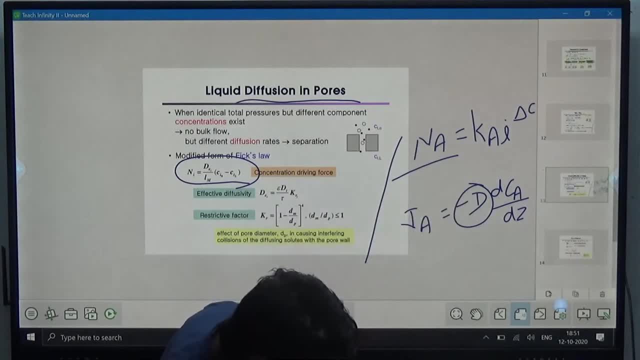 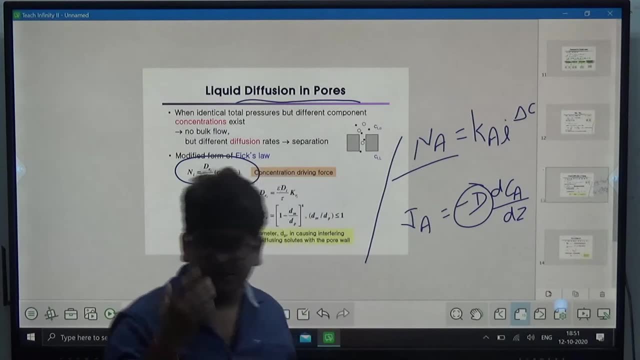 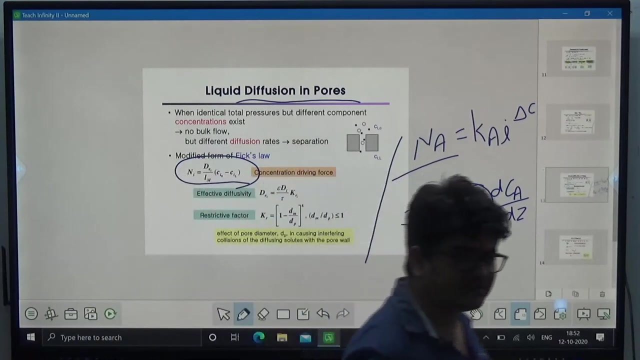 Thank you guys. See you in the next class. And yes, one more thing: if you have any doubt regarding membrane separation and the practice questions, you can join the telegram group. I will share some practice questions. farewell, MCQ type questions regarding membrane suppression. till tomorrow in your group. 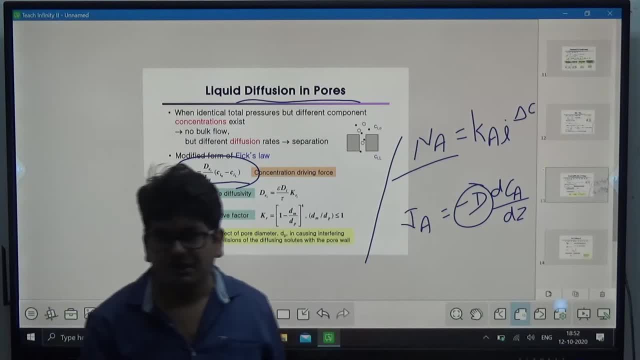 The questions are ready and we will share one- you can say assignment- regarding the membrane suppression in the telegram group. The link will be available in the description so you can join that.